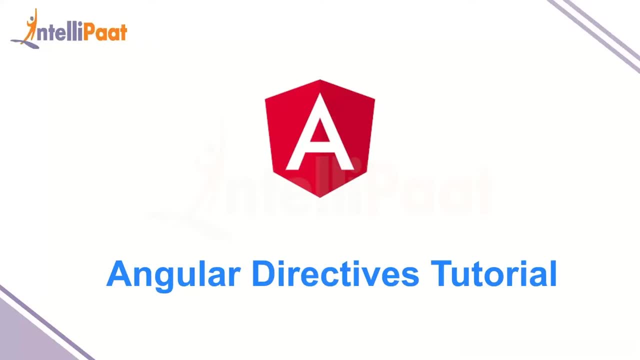 like to ask you to subscribe to our youtube channel. click on the notification bell icon so that you never miss another update. click on the like button if you liked this video and put in the comments section below what other technologies you'd like for us to cover next, and also if you. 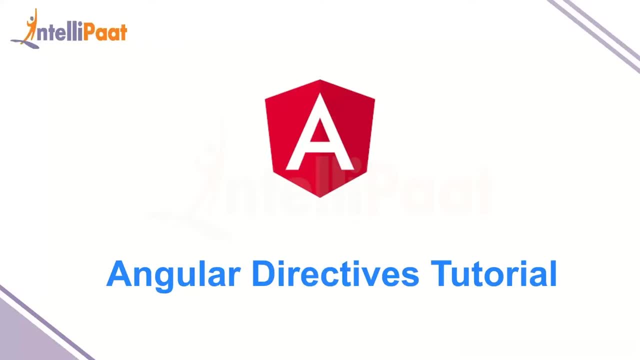 have any questions during the entire presentation, put them into the chat box and our team is there to help you out with any questions that you might have. and if you think any of the technologies and the code that we're writing right now is a little difficult or advanced for you to understand, uh, do. 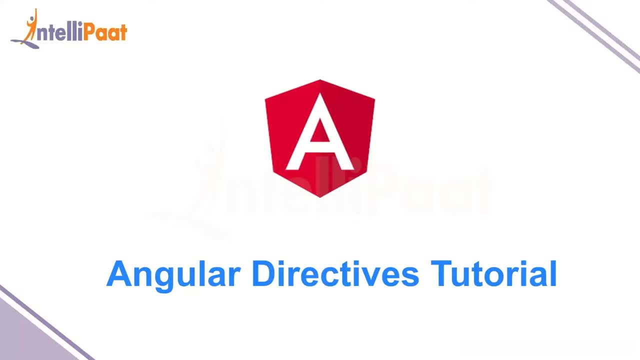 not worry, at the end of the presentation we'll guide you through some of the resources that can help you out into learning these things. so with that, let's take a look at how we can use angular directives. by taking a look at the agenda. we begin by taking a look at what is an angular directive. 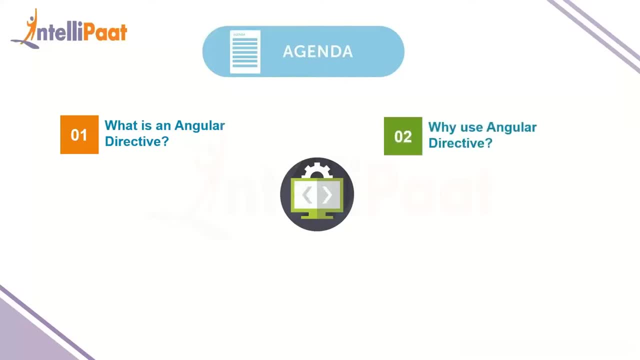 an angular directive is the core of what we're trying to discuss here, then we'll take a look at why should you use an angular directive. it's not necessarily the case that you have to use an angular directive. however, an angular directive provides certain features and makes it easier for you to get certain tasks accomplished. 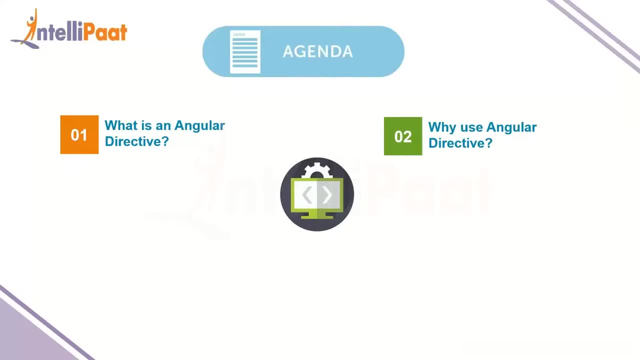 we'll take a look at how you would use them, but before we have to understand why would you want to use one? what does a direction do? then we'll take a look at the types of angular directives available. in angular there are three types of directives and we'll take a look at all of those. 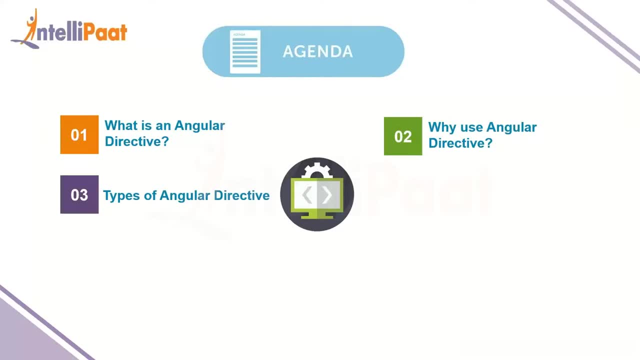 we'll try and understand which one suits best your need and why one might be more suited for your current scenario than the other. finally, have a hands-on in which we'll try and create and use all different kinds of directives that we have discussed in the previous slide. so we'll discuss the types of directives and 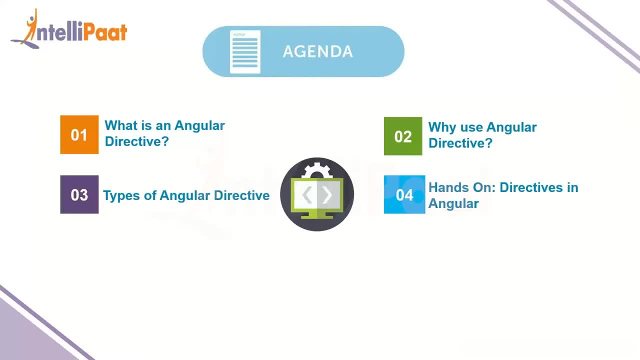 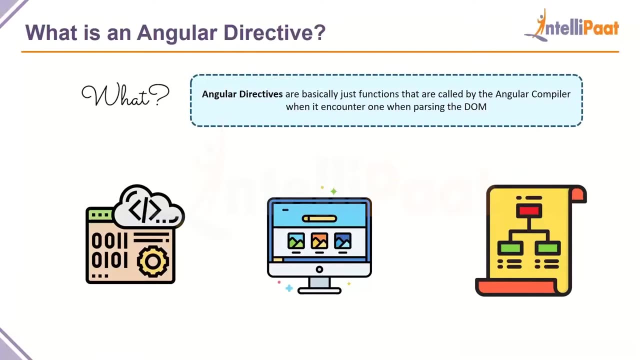 then in the hands-on, we'll show you through code how you can use those. so let's take a look at what is an angular directive. so angular directives are basically just functions at the core. they are just functions in angular. since angular is a framework, it allows for you to add certain bits. 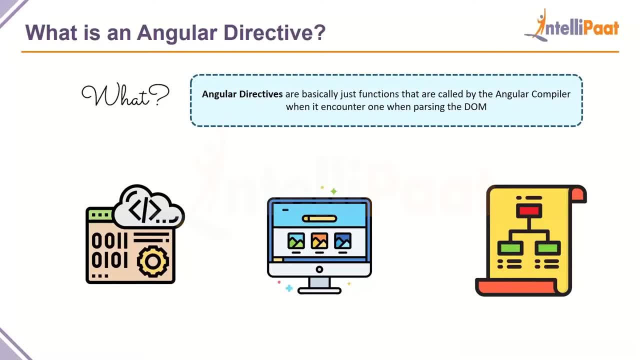 of code to manipulate its behavior or its default behavior. in this case, if you want to create a directive, you firstly have to create a function so that function gets called by the angular compiler when it encounters one or one parsing the norm. so in case you're not familiar, 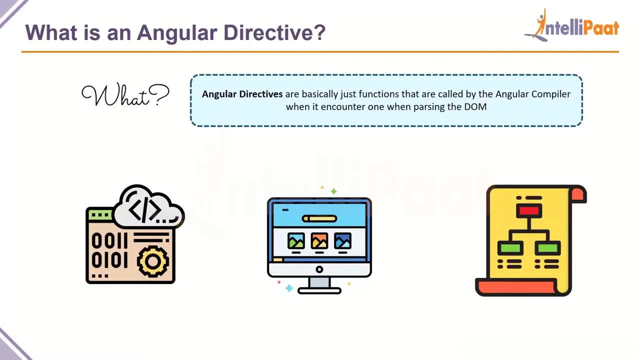 the way things work in angular is that you define your your bits and pieces of code, ranging from your templates to the code that is behind the component and everything else. you register it with your module, export that module and make it available to your application. finally, when the 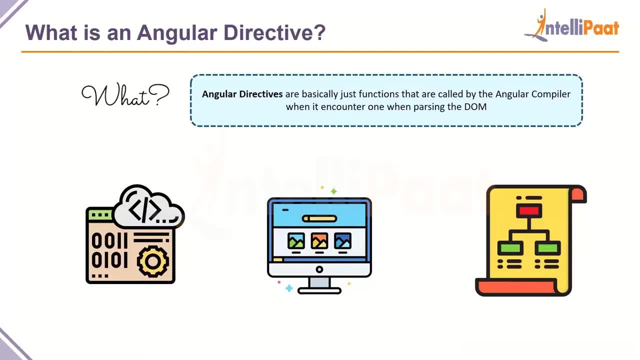 angular compiler runs, it starts with the app module, and then, when the compiler runs, it starts with the app module. and then, when the compiler runs, it starts with the app module, and then, when the starts building a graph of everything that it needs to compile, ranging from the templates, 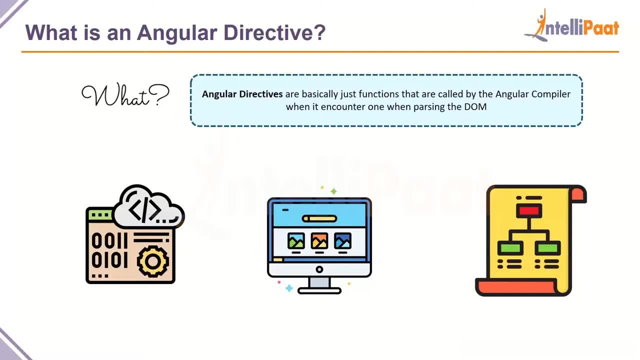 css files, images, html code, transpiling the typescript code and many of the other things that it needs to do, and during that time, it encounters certain directives. so, as we have already discussed, the directives are just functions, so what happens then is that they will take a look at the directive. as soon as they take a look at the directive, the compiler will 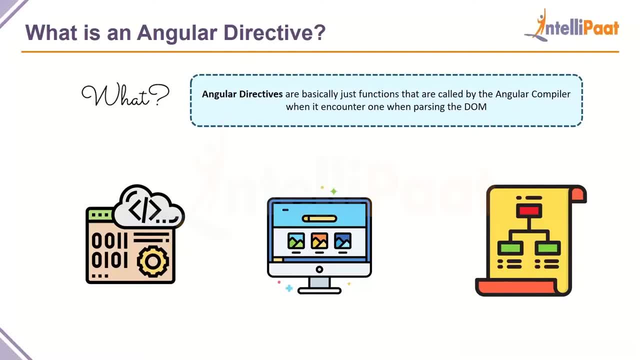 figure out that this is a directive that has been registered by the user. it has a special meaning for me, so I have to execute the necessary function with that directive in order to figure out what the value of this html component should be. so the direction gets executed, whatever the value. 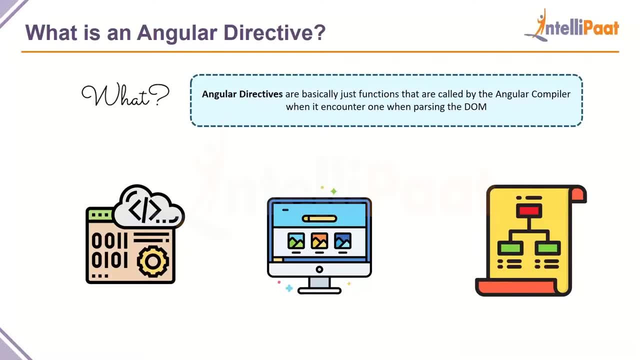 is there, then it gets, uh, substituted for the original value and we move ahead. so that's why directives are useful, because they allow us to basically define functions that could add some dynamic applications to our application. now, with that, let's take a look at why would you want to? 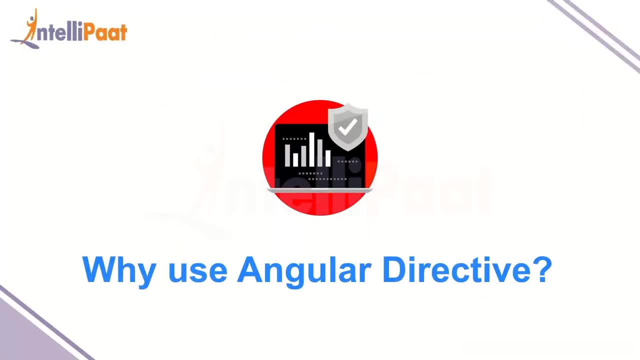 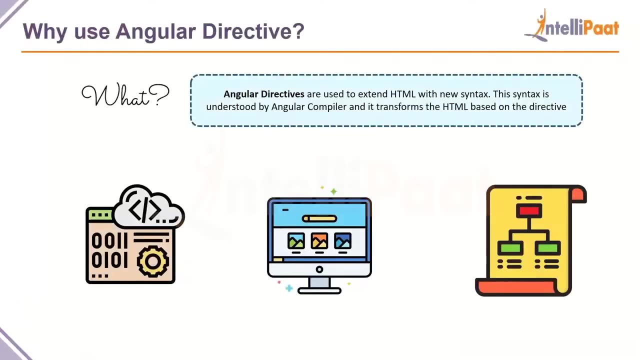 use a directive, you know that they are just functions that we could add to our applications that allow us to perform certain tasks in angular. but what kind of tasks and why are they useful for us to perform in this way? well, angular directives are used to extend the html syntax. 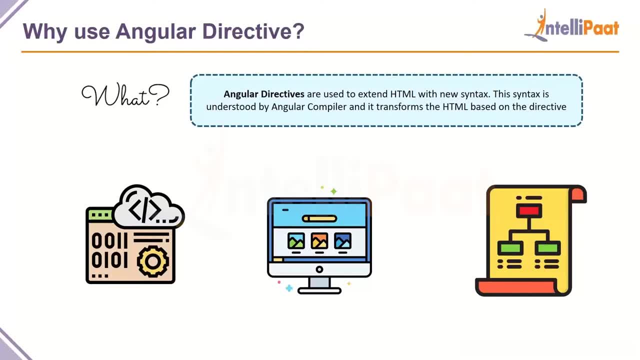 with the new syntax. this new syntax is understood by angular compiler and it transforms the html based on the directive. to give you a specific example, given that you have fetched some user data from the internet, let's say that you are trying to build a social networking site in which 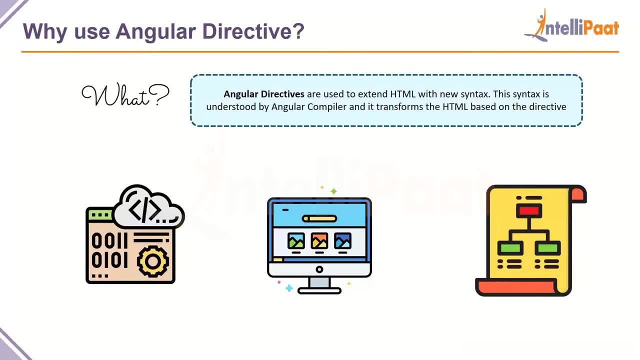 a user can follow the users. now, in scenarios like this, you have to create a list of users that the user is already following or a list of users where the user is not following those users but can follow those users. suppose i search for some name and i get a list of those users now when i search. 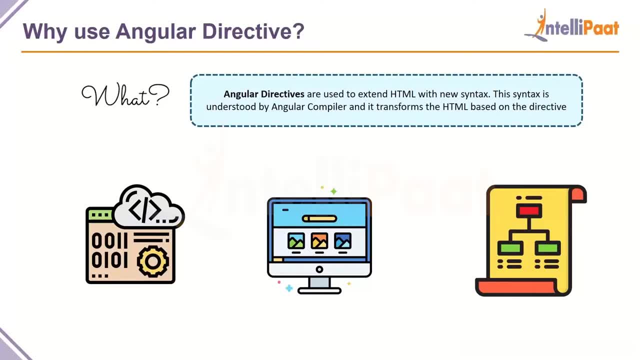 for those names. the way it happens is that i will contact my backend server, the backend server will return me back the the data points that i need in order to build that user interface, and then i have to show it to the user. in scenarios like this, directives are useful because all we are doing in this scenario at 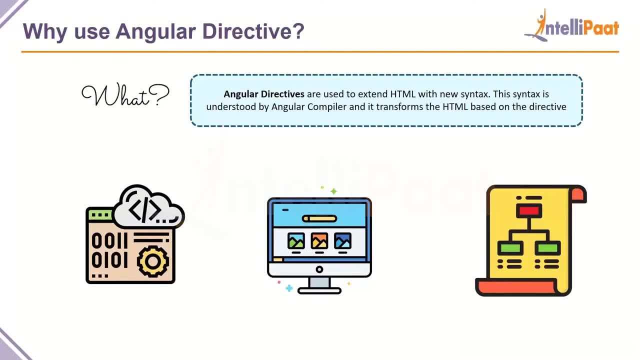 least is that we are looping over all the users that have been sent back to our sent back to us by our backend server. so that's basically the idea behind using angular directive: that we are trying to manipulate the html in some way or the other. we're trying to manipulate the template. 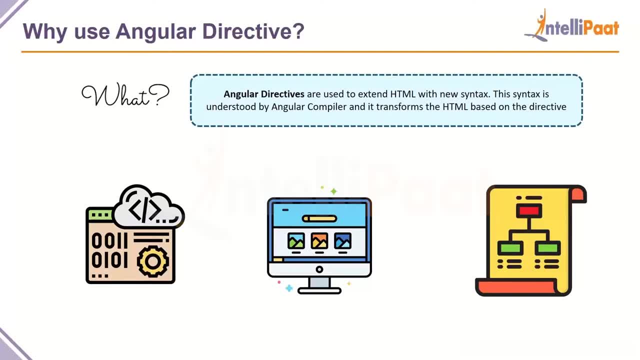 we're trying to add some new content, change the structure of the content. we're trying to add some styles to it. we're trying to add some custom behavior to it, whatever it might be, and all of this is done using directive. directives allow us to extend the html syntax so that the angular compiler can understand it. now these directives need to be. 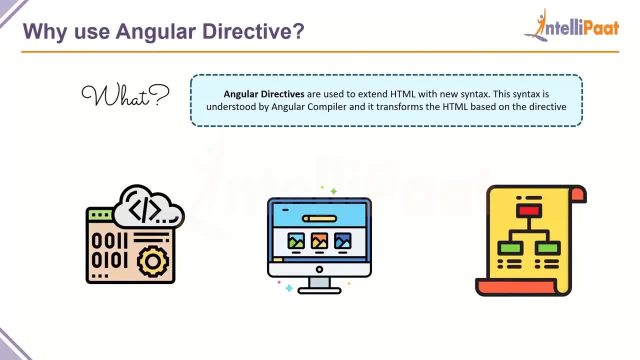 registered with angular as well. so if you create a directive yourself, you can't just use it offhandedly. you have to register it with angular compiler so that when the compiler comes along the directive it understands that. okay, this is not some new html syntax, this is something that the 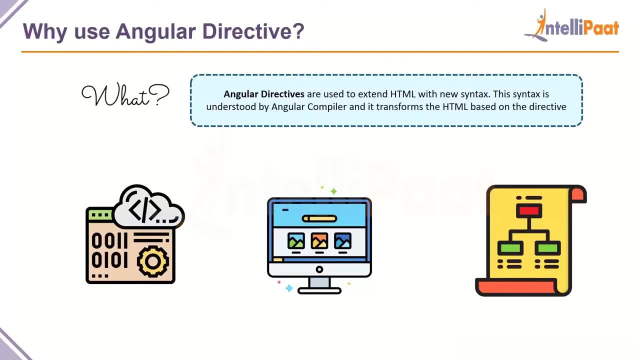 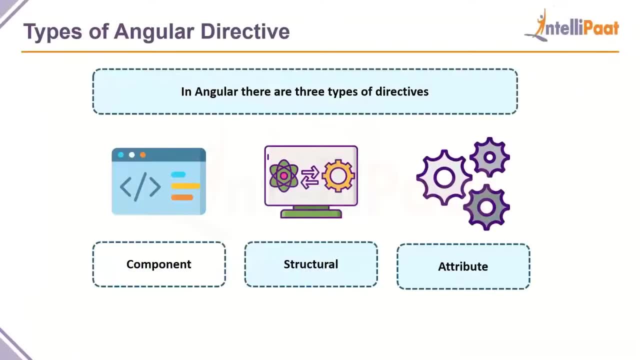 user wants for me to fiddle around with. so keep that in mind when you're trying to build new directives and work with directives as a whole. then comes types of angular directives. uh, in angular there are three types of directives. there's also a custom directive, but that's not really a 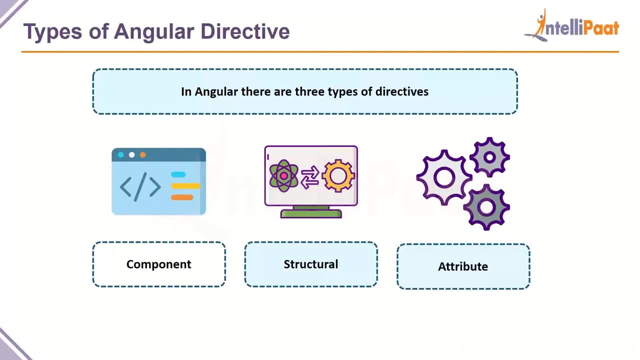 type of directive. you can create a custom directive on your own. the three types of directives are component, structural and attribute. let's discuss them one by one. firstly, we'll discuss components. in case you have ever worked with angular, you know that when you're building a user interface, 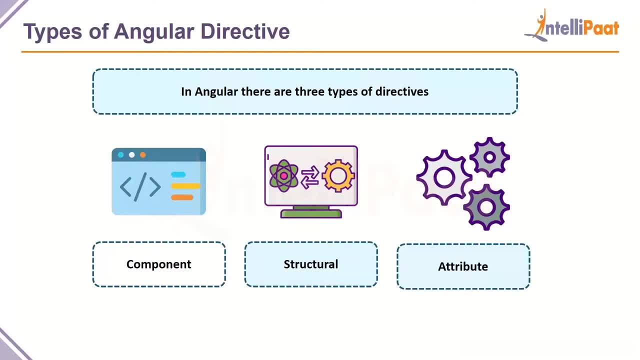 you need to generate a component. that component's job is to define a really small piece of the entire user interface. it could be a list of users. it could be a list products. it could be a description of a single product, with its price, its image, buy button and many other. 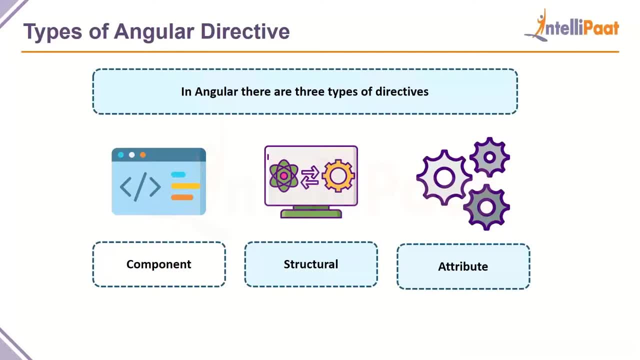 kinds of things. so this is why angular is new and has been completely rewritten from angular js: because they wanted to introduce the concept of components, because that makes it really easy for developers to build their applications. now you build a component. in that component, you put in everything that you need. 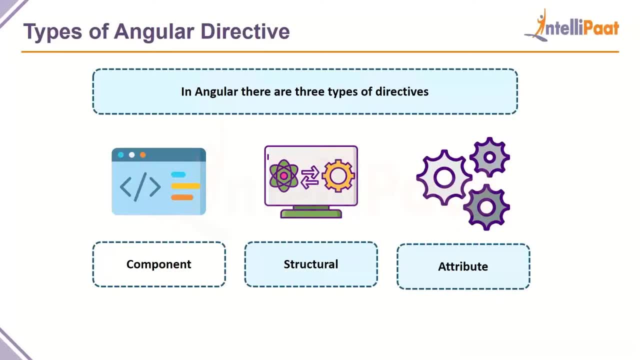 for the user interface to work, and then all you have to do is the selector that you have defined, you put that in the html and that's it. that's how the entire component works. the component itself is a directive. so when you are adding new tags in html, which html has no clue about, 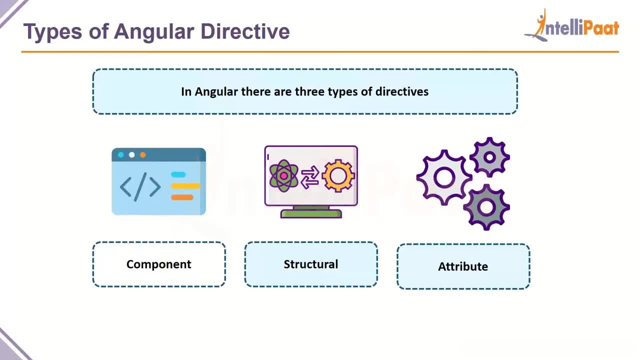 what they might be. angular compiler takes a look at the code, replaces that tag with the entire template and styles and the behavior that is needed for that component to work. so that's why it's called a directive, because it is changing the html context. then comes structural. 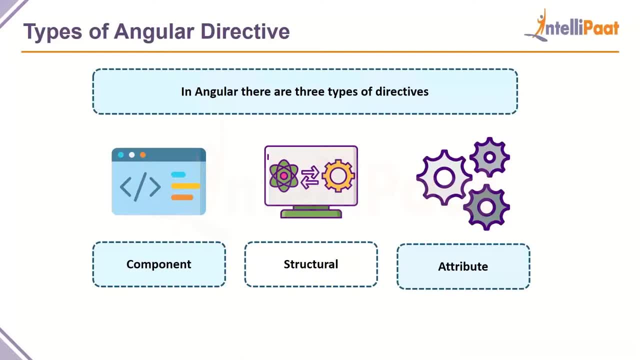 so in component, we were adding new content, but in structural, what we are doing is we are trying to change the structure of the content. so, as we discussed in the previous slide, when we're trying to discuss why would you want to use an angular directive? one of the reasons that i gave was when 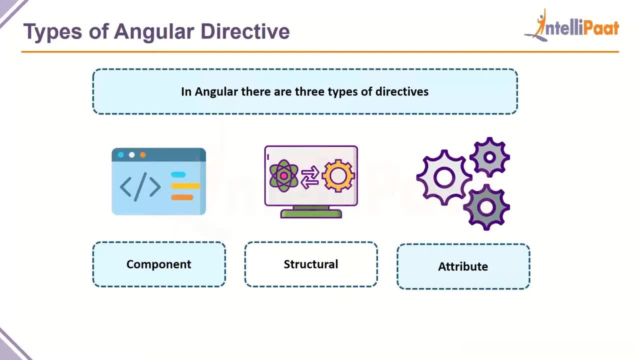 you get some dynamic data back from the server and you want to update the component, you can define it and as in terms of directive, and that will work. so similarly here also, let's say that i have a list of names that the users can uh, that the user can see. 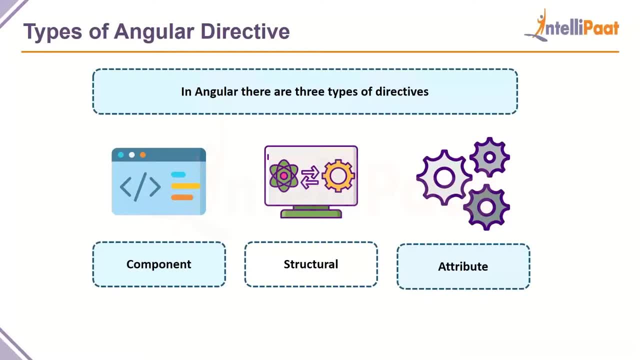 or a list of users that the user can see. what they can do is get those username from the server. this takes a bit of time. after getting that from the server, i then publish it onto my users followers page or suggested followers page. now, in scenarios like this, what is supposed to happen is: 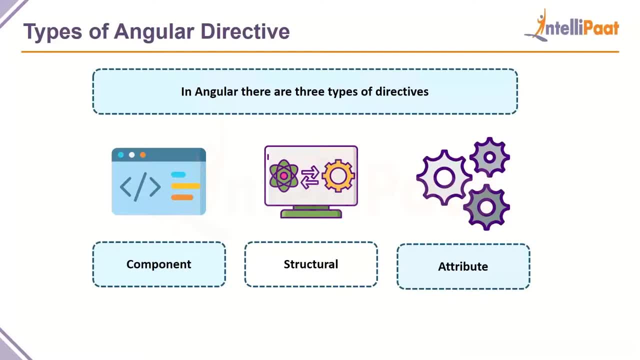 when i populate the data i want to loop over. all the users generate new bits of html and insert it in places where i need them to be. so this is where structural directives come into place. they are not just there for looping over stuff, there's also ng. 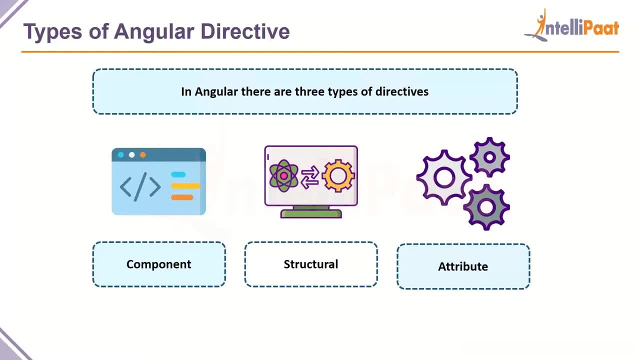 uh, there's also directives that can allow you to show or hide a particular content based on a particular value of a particular attribute. so let's say that the user has clicked on a checkbox that says show me suggested products and you want to only when the user has clicked. 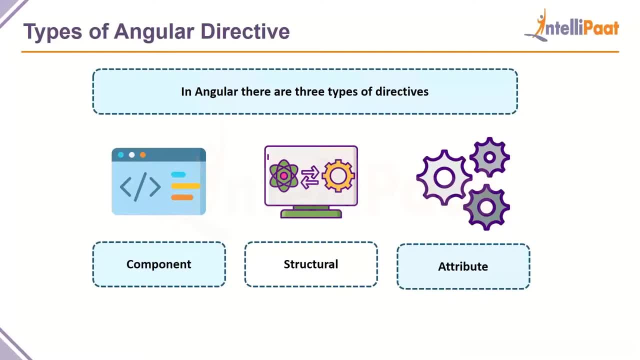 on that checkbox, you want to show the suggested products. well, that way you can just keep track of a variable and use some structural directives in order to show or hide some data. so that's what structural directives do? they change the structure of the component that we have already shown to the user, change the structure of the. 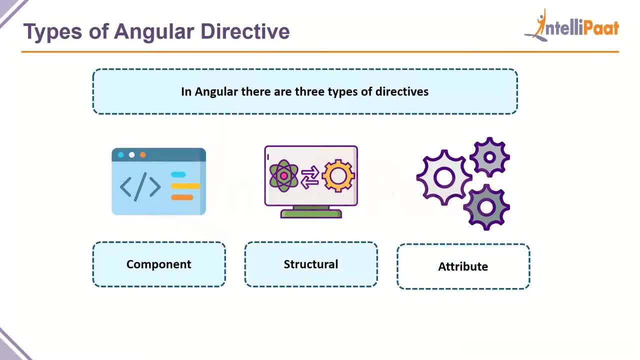 template and then comes attribute. if you have ever worked with html, you know what an attribute is. in basic terms, an attribute is something that changes the behavior or the appearance of a tag. so, for instance, if i have a tag, let's say h1, and i want to change its style, the style attributes can be used here, although you can. 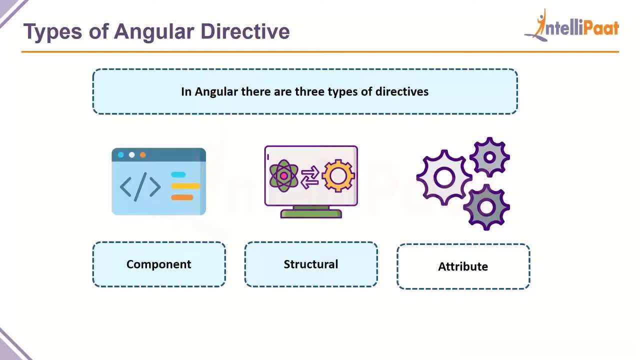 still use css as well, but you also have the ability to use your style. similarly in the attribute directive, what we do is we apply or remove certain styles from our html code or certain attributes from our html code. so if you want to add a class, we want to add some styles, we 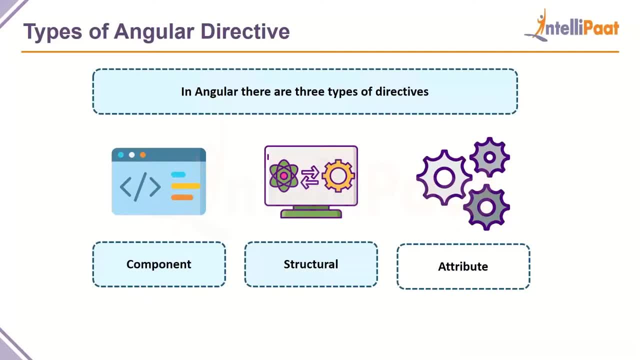 want to do something else, we can use attribute directive. attribute directives are really used well because they don't let us muddy up our html code. all they allow us to do is to add new attributes to our already existing html code, so that's a really nice way of thinking about that. 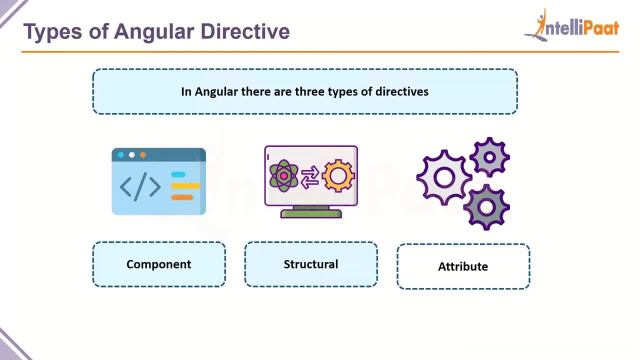 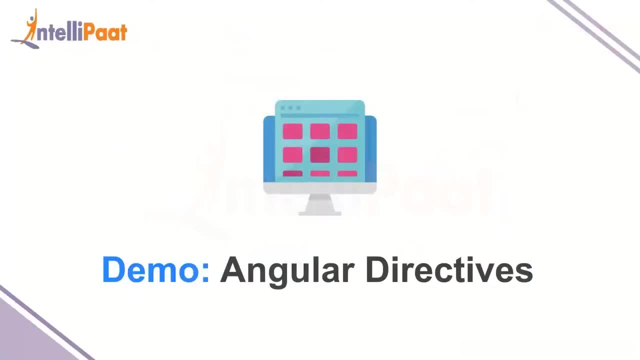 so we have discussed the three kinds of directives that we could use. we discussed components, we discussed structural and we discussed attributes. now it's time to take a look at these directives. to follow along, you would need to have installed angular cli. in case you don't have it, you can still follow along with us. you would have to open up. 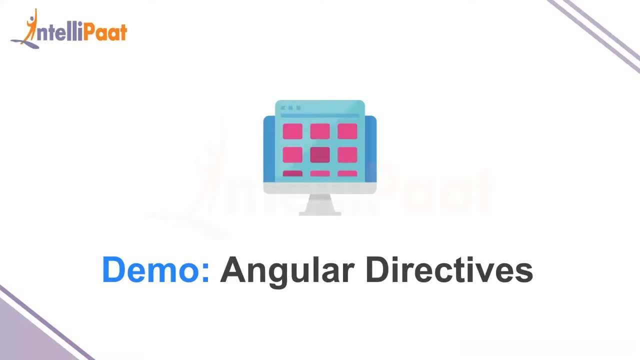 an online editor at stackblitzio. create a new angular session there. it's free, you don't even need to sign up- and then you can follow along with us. if you have angular installed, then let me show you how you can create a new application and then serve it so that it can be used so. 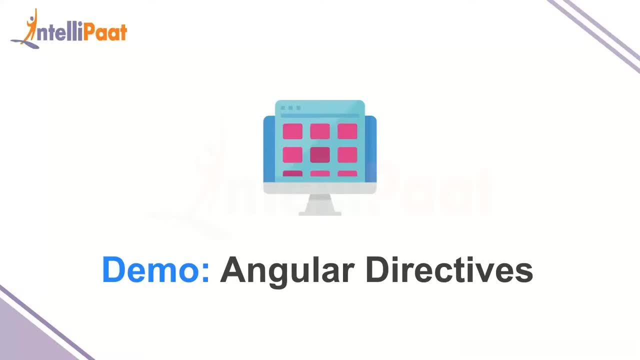 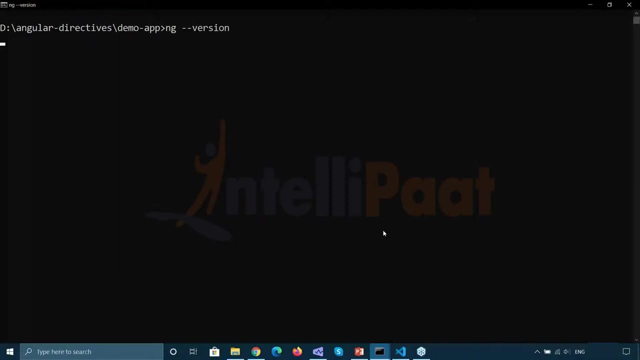 i am going to go out of the presentation now. let's take a look at what we can do. so i already have generated the application, but to show you how you can do it, open up your command prompt. make sure that you have typed the keyword ng. take a look at the version if it shows you that. 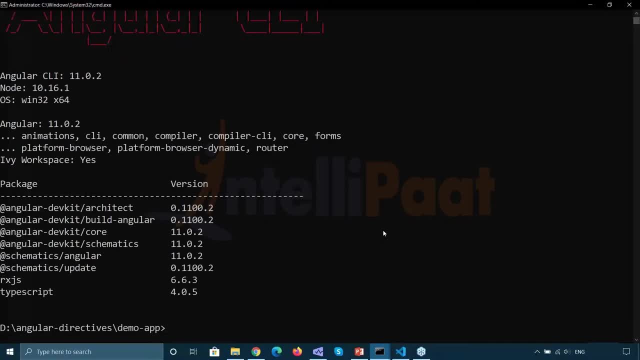 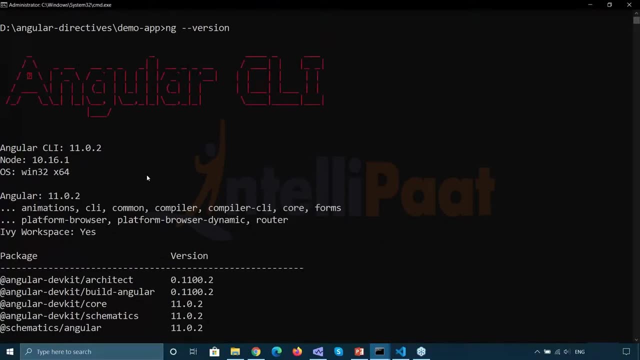 ng is not a recognized command. that means that you have not installed the angular cli and you are not ready to create your entire html, entire angular application. i have the angular cli version 11.0.2, which i believe to be the latest version, but you can choose. 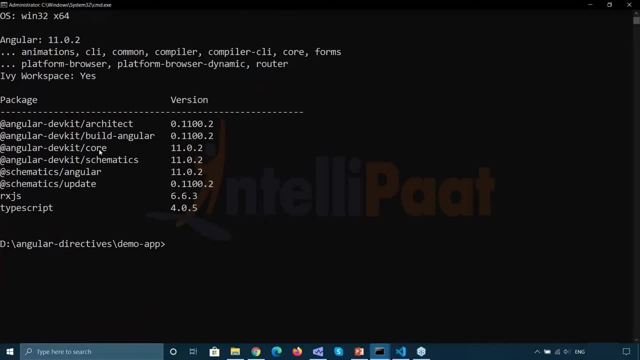 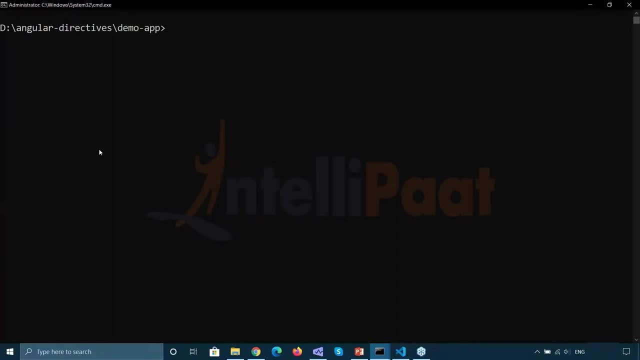 whatever version you wish to prefer, it just needs to be able to generate some components. so, after this, go to a folder that is completely empty and you want to create your angular projects there. all your angular projects can live in that folder. to generate a new, new project, you type in ng new, new means. it's generating a new project. 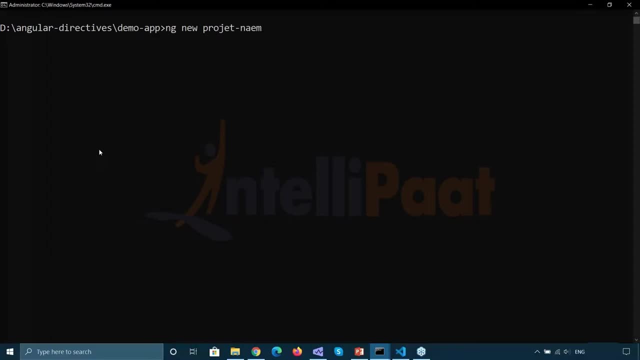 and then you can give it your project name. uh, in my scenario, i have given it the name of demo app, demo dash app, and i can press enter. now i already have it generated. it's going to take a little bit of a time and once it starts generating, it will ask you a few questions. 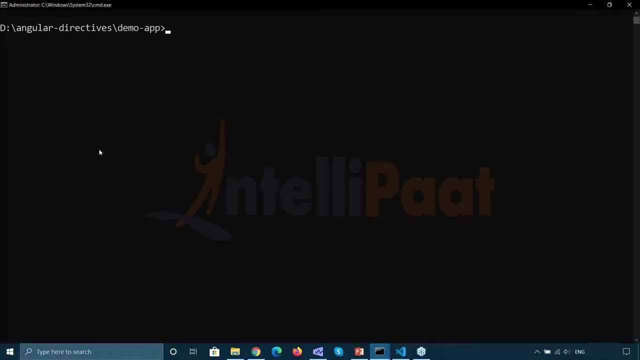 so you want to enable strict typing. so when it asks for enabling strict typing type, yes for y and press enter, then it will ask you for if you want to include routing in your application. you are not going to be using routing, so press n and press enter, which means you are declining the 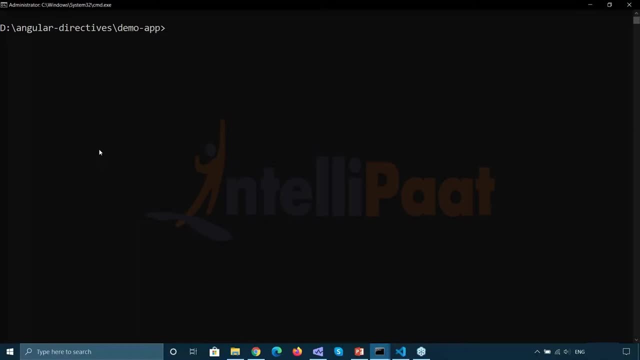 that option. and finally, it asks you what kind of a style processor- pre-processor- you wish to use. do you want to use css? do you want to use sas, sdss, less, whatever? so just select css, because we're not going to be doing much of styling in this. uh demo and press enter, then it will create all the files. 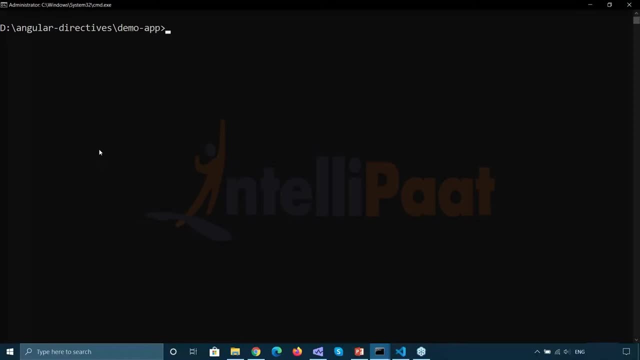 it needs to create and then it will download all the node modules that it needs to download. this will take a little bit of a time, so don't worry. once the node modules are downloaded, it will show you that everything is working fine. you didn't need to cd into the demo app folder. that. 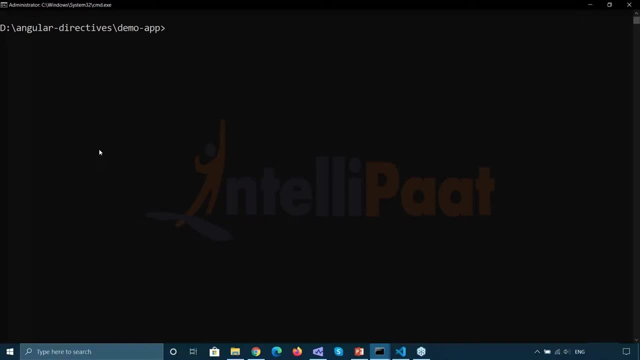 means you take your command line session into that folder and now you run, uh, the command that says ng. so or if you don't want to type the entire command, you can just type ngs. angular will understand. you will press enter and this will start up a command. uh, a server, but that command. 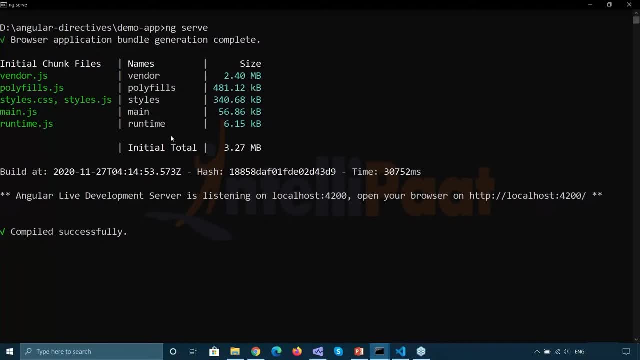 line session will then be completely taken over and you can try it again, anything on this. this is what it will look like after you type ng sir. it will generate the entire bundle by compiling everything that is that it has, and it will show you the size, show you the hash. 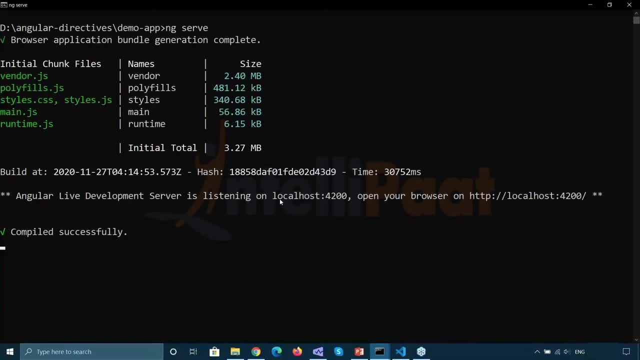 and it will tell you the location or the browser location that you can go on. uh, you can go on local host, colon 4200. it could be a little different for you depending on the port that is available, but by default, mostly it's going to be this. when you open it up, it looks like this and: 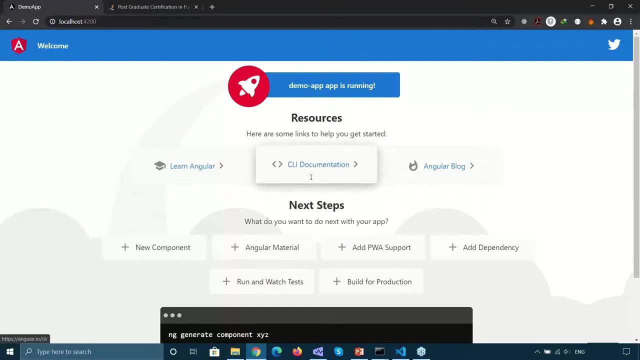 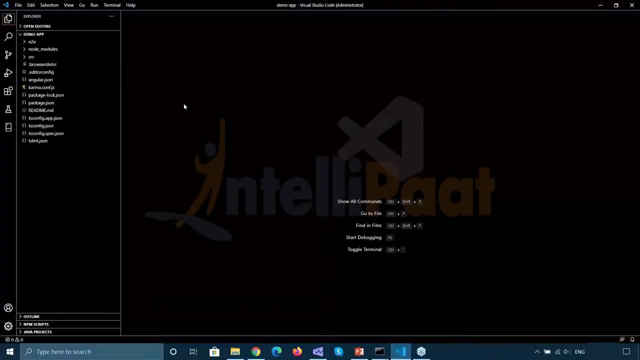 it's quite okay, but we want to now go into our directives folder, so since i named it demo app, it's going to call it. demo app is running now. if i open up my code in my code editor, i'm going to be using visual studio code. you can use any text editor that you want in order to make the changes. 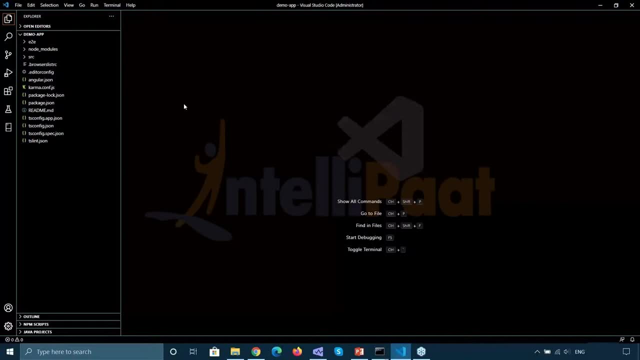 these changes are going to be automatically picked up by the angular cli and it will compile the new code and show you if any errors are there and you can run along with. now let me just show you how it works right now. we have one component. that component is called the app component inside the 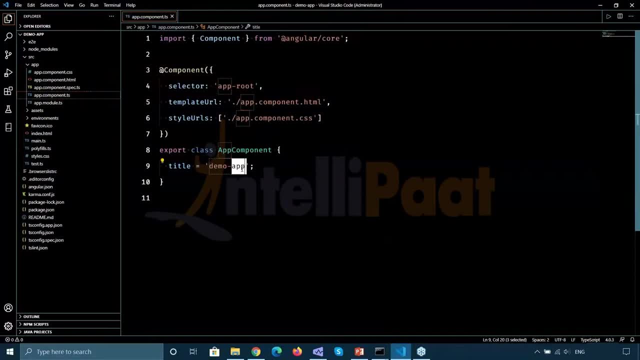 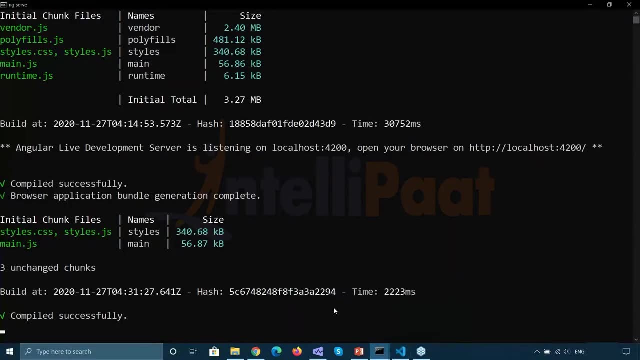 component. we have some typescript, that title that is called demo app. i can change it. i can call it demo app location. i save it, as i told you that this will compile automatically. so, as you can see, this is recompiled and now, if i take a look at this, it will rerun this entire thing. and now it's. 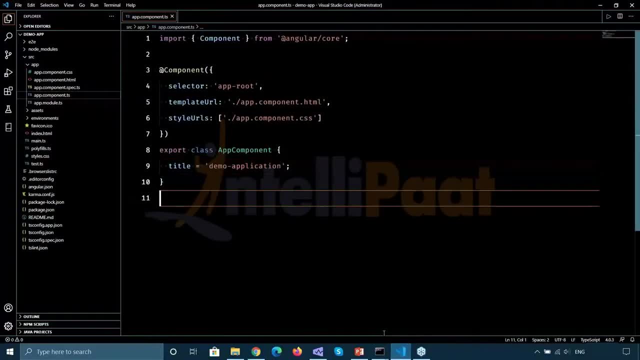 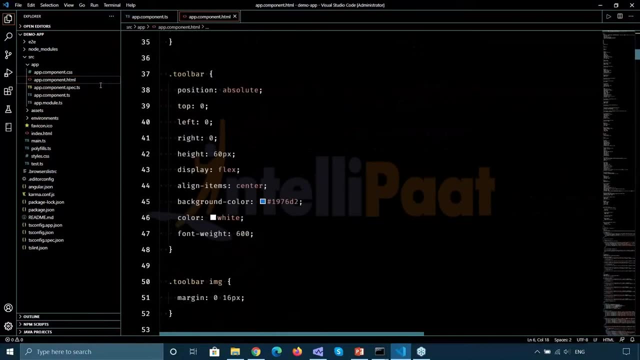 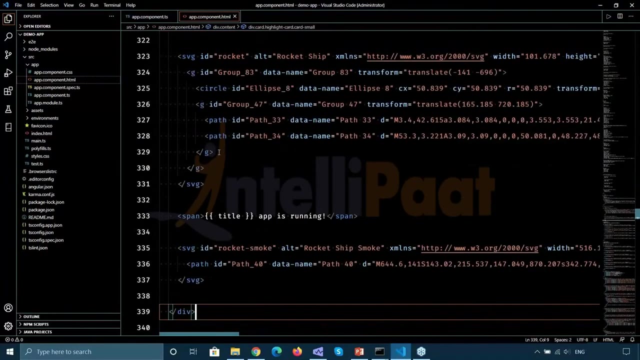 called demo application is running, so now you know how it works. the way it works is that it takes a look at the title html component. uh, this is the styles that have been added to the components. uh, template directly. we need to scroll down a little bit, yeah, so this is what it looks like and, as you can see, this is. 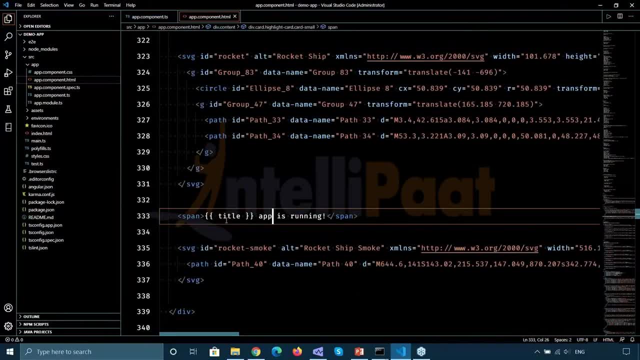 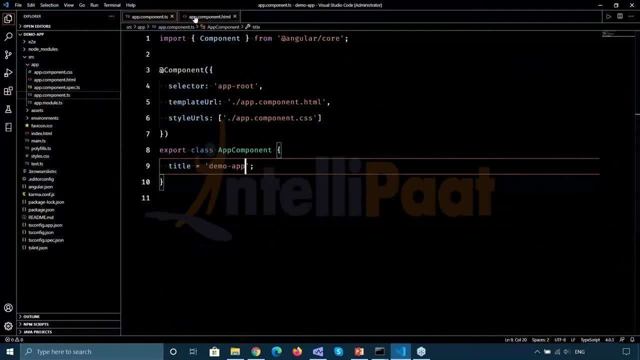 interpolating the title, so this is done as well. now it's showing that the title app is running and the value of the title we have changed to be demo application. i'll just change it back to demo app because that's what the default was. so now that that's the way it works in the app module, it 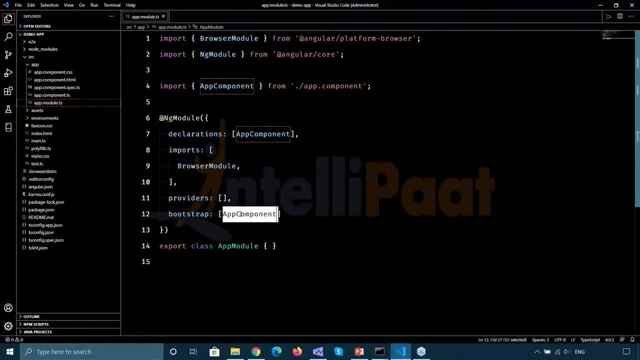 tells the uh module that, okay, the entry app, the bootstrap component, the component that needs to be displayed right at the beginning, is the app component. so it will take a look at this and understand: okay, that's the component that i want to use, and it will do that. now that that is done, let us do a few things. let 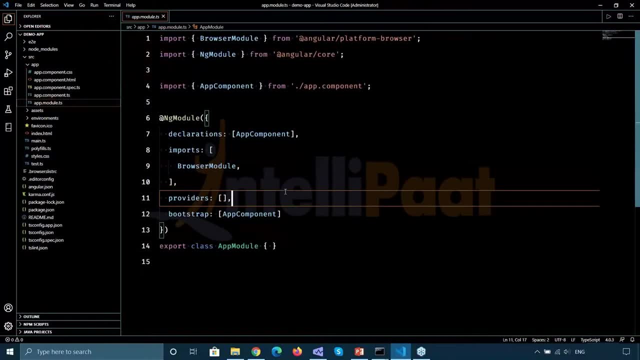 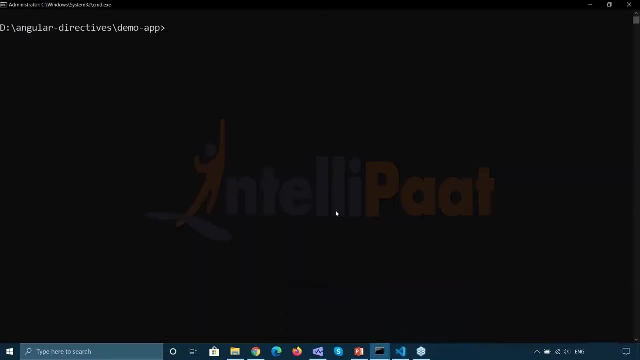 us try and understand these directives one by one. so the first directive that we had talked about was a component directive. to create a component i have to go to the angular applications directory. i have to type in the root directory i will type ng generate if i don't want to type the entire word. 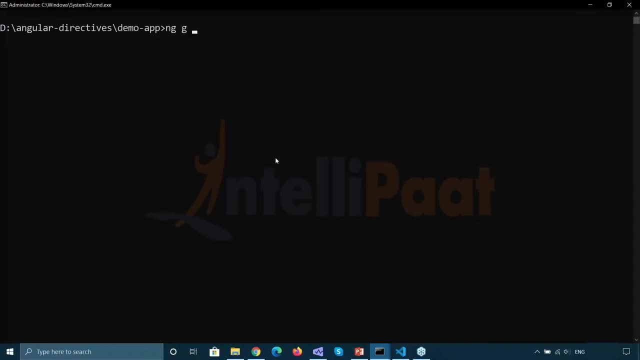 i can type just type g and angular cl. i will understand and ng generate. and i want to generate a component, so i will type c and now i can type the name of the component. i'll call it names, n, a, m, e, s or i can also call it users component. i will press enter. this will take a little bit. 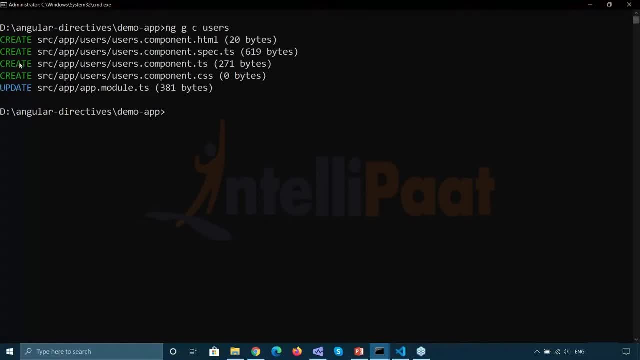 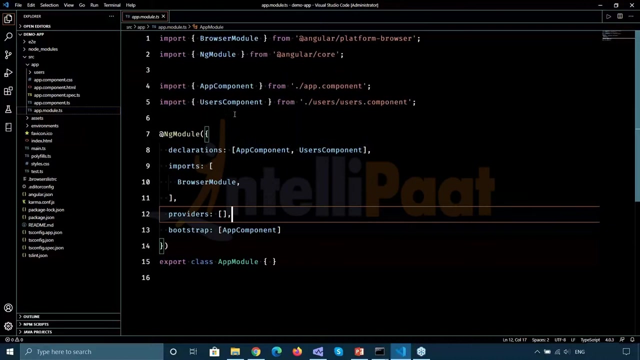 of a time it will generate a few uh files. as you can see, it created four files inside the users app slash users directory and it updated the appmodule ts file. if i open it up, you can see that earlier there was only app component, now there's user component as well. angular did. 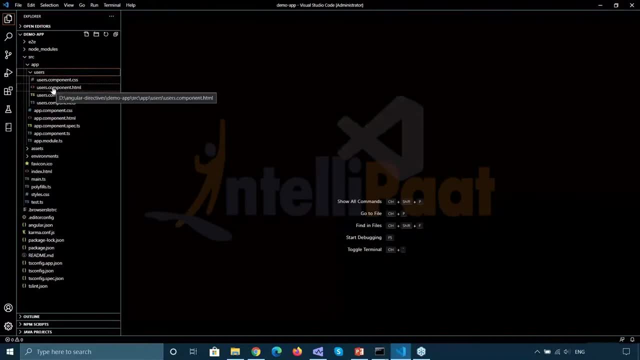 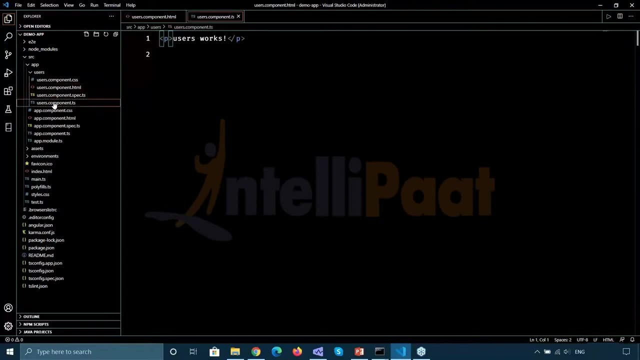 that for us, or the cli did it for us. now if i go back, i take a look at the components html, it's just showing users work. so this is the name of the component and this is the tag, and i go open up the code. now let me just change the main main component from being app component. 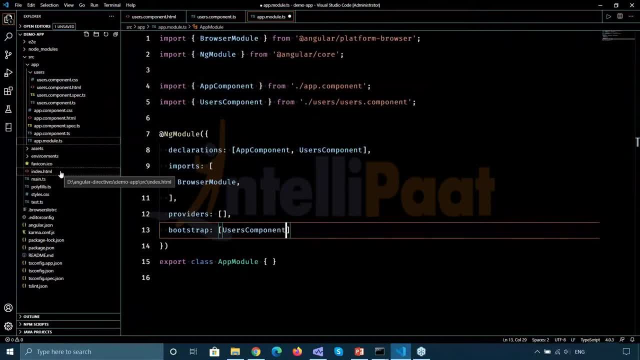 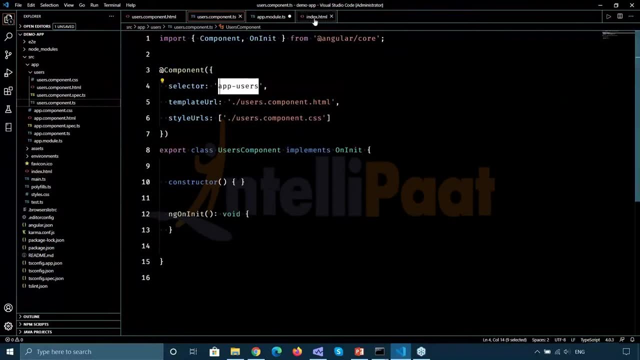 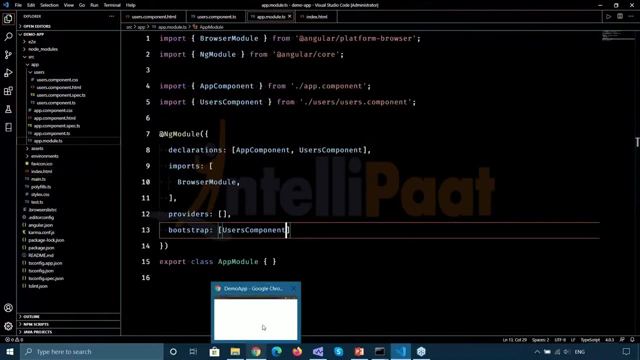 to users component and inside html, i have to change this. as you can see, the selector here is app users. if i were to change this here, save this here, save this here. and if i go back to my demo application, it shows users works. so why did this work? well, the way it happens here is that. 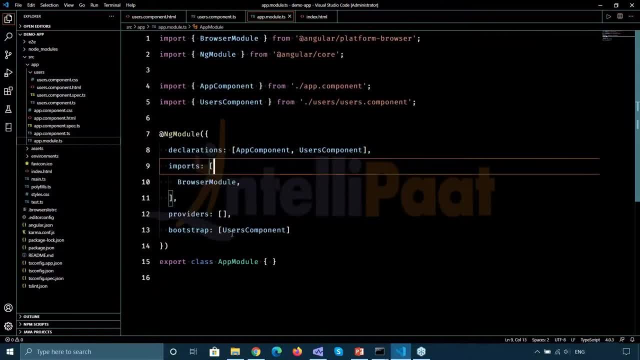 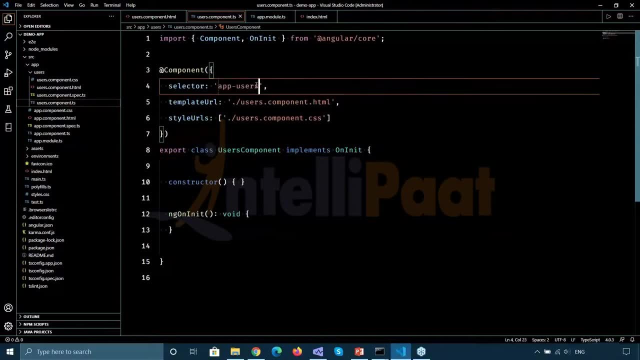 the application gets recompiled. it takes a look at the first component that it needs to compile, which is users component, opens it up, takes a look at the selector, registers it and tells angular. whenever you see this tag being opened and closed somewhere in your entire html templates, you have to understand that this is an. 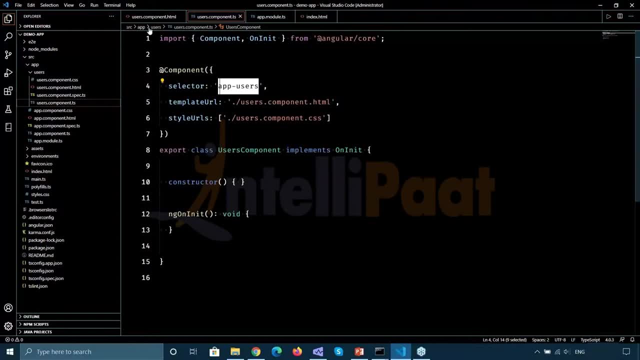 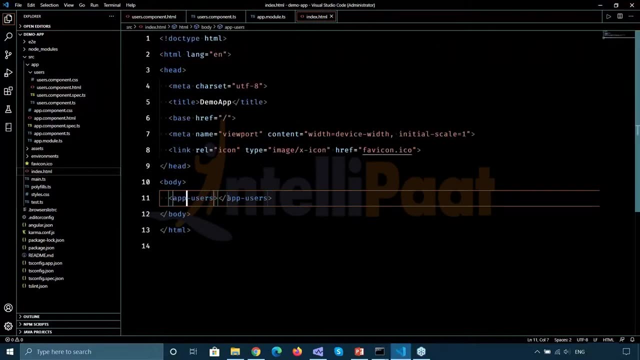 angular component and you need to replace this tag with this html. so angular compiler opens up index dot html. takes a look at this tag, figures out that this is a tag that i have already seen. i can't skip over it. i have to change it, and then it changed. 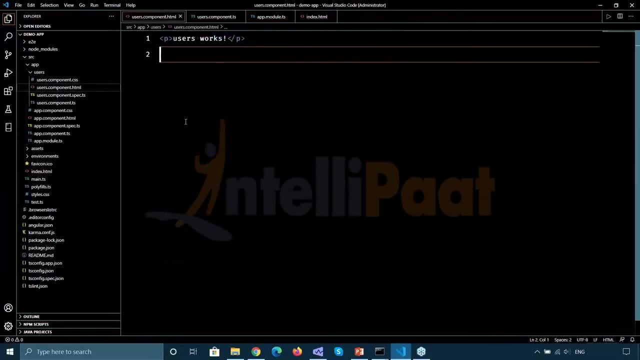 that changes it to the HTML component that we just saw. So that's how the component directive works. Now let's take a look at the structural directive Now. inside my users component- I have no data right now. Suppose I wanted to create a few users. 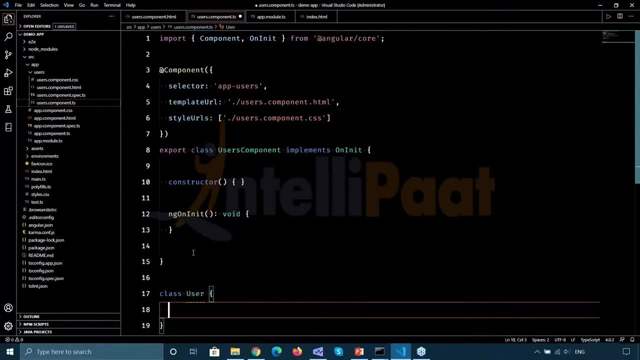 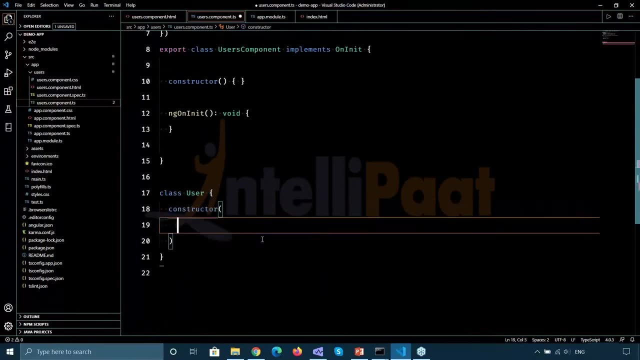 I'll create a class named user inside the user class. I want to create few properties, So I will use the constructor inside the constructor. I will type in private underscore name. and why I am typing underscore I'll show you in a moment. 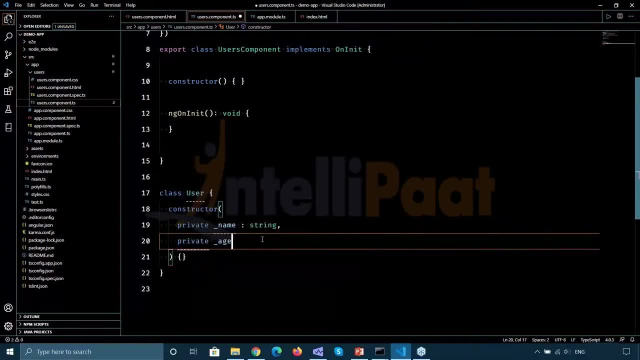 This might be something that you might not know, So you will take a look at this, and the age would be a number. This is what TypeScript allows us to do, So with that, I want to create a few getters, If you're following object-oriented programming. 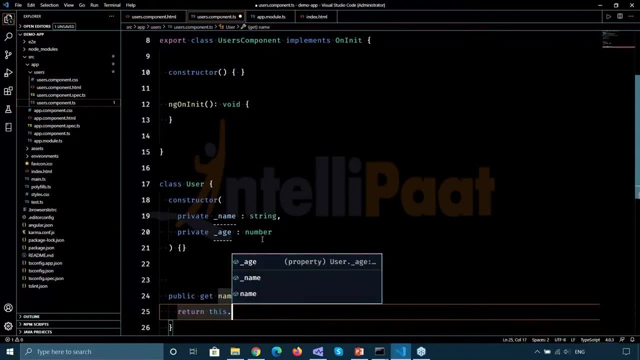 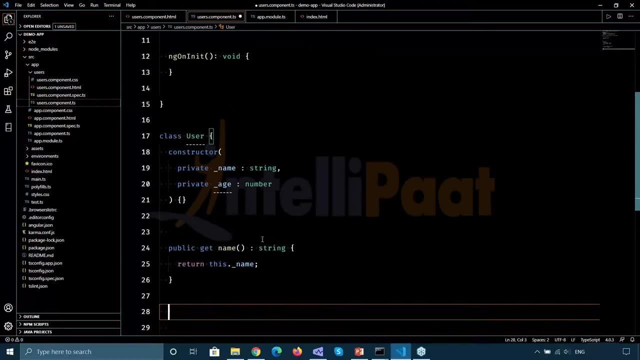 you know that getters are important. Getters basically mean that if the user is trying to access some property of my class, I want to give it to them, But after some processing. Here no processing is required, So I'll just do it this way. 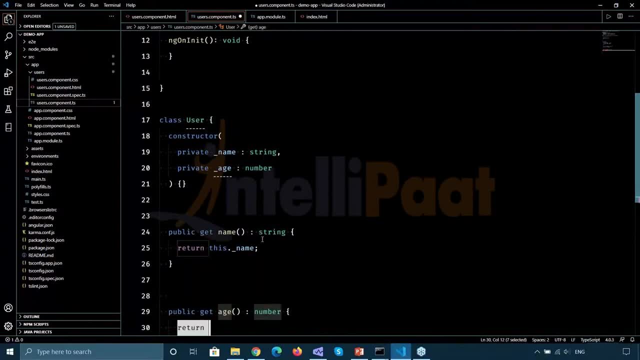 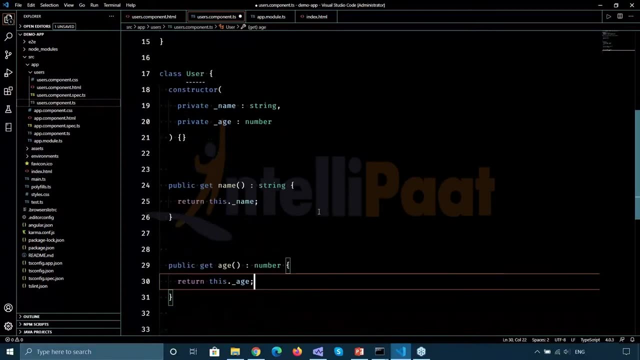 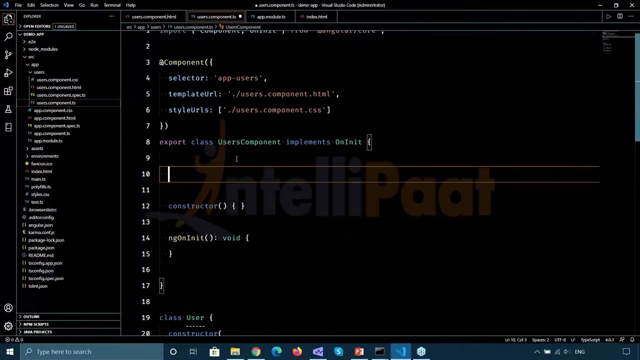 and Visual Studio code helps immensely. Number and again, this dot underscore age. So now I have a user class, I have age and name property on it. Now all I have to do is I have to create a few users So I can do it here. 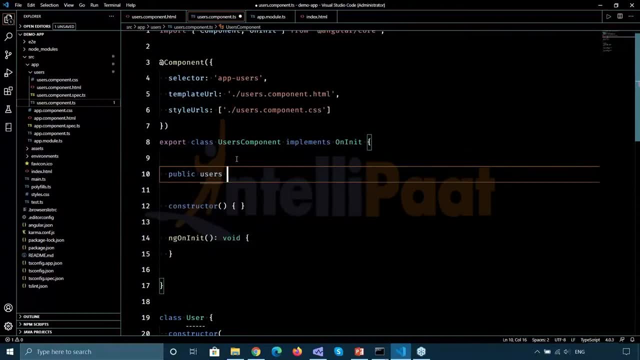 So I will just create a public users property of type string array of user. What it's going to do is I'm going to create a new user in the user array, I'll create three more users. So, as it's TypeScript, I can see what I want. 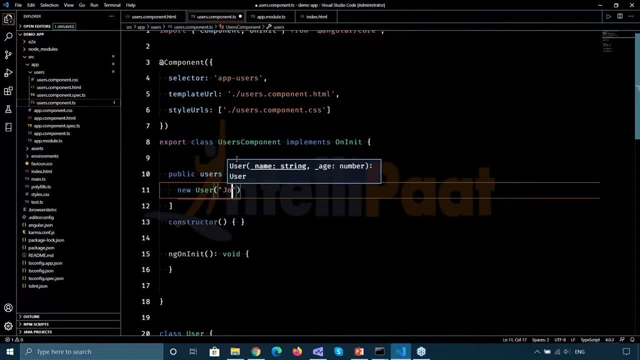 I want to pass in a name and an age. name is to be a string. So let's say John. age is supposed to be a number, Let's say 20.. I'll create three users: John, Jane, John is, age is 23.. 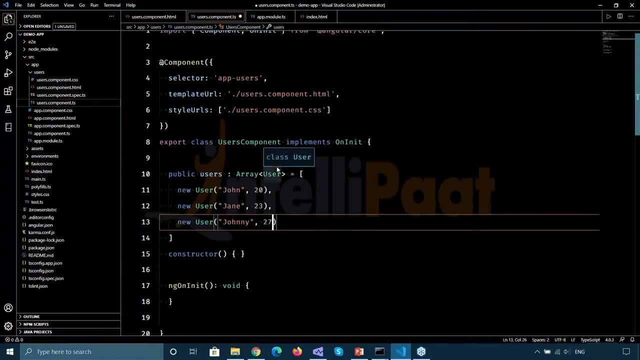 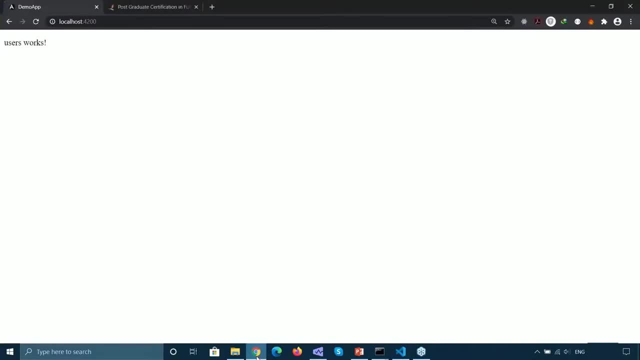 His age is 27.. Now this is done. And now, if I save this, it's going to work completely, because nothing has changed. If I go back to the code, it would reload, But not since nothing has changed. Nothing will work as of now. 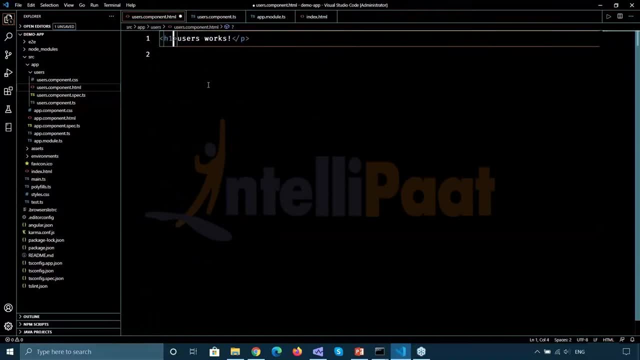 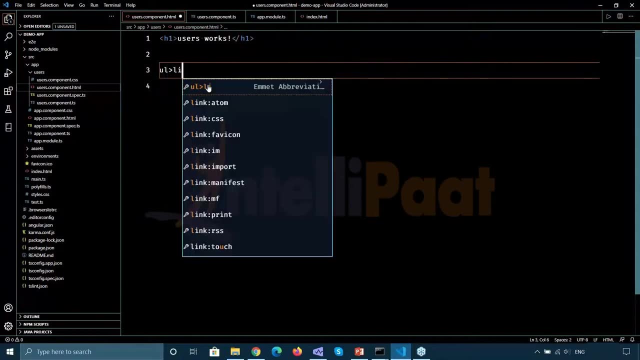 If I go back to my users component Now I want to: firstly, changes to H1. H1 is to be the new heading and now I'll create an unordered list with a list item and that list item is going to be repeated. So here's where the structural directive comes into play. 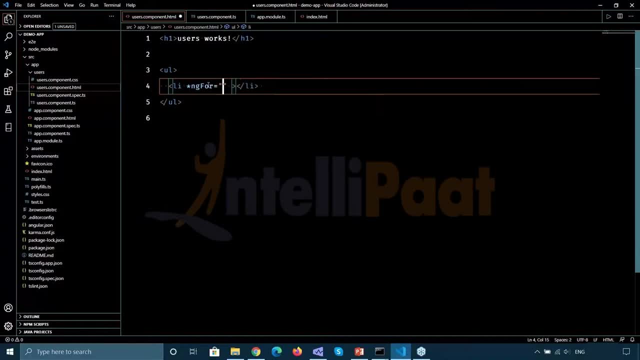 I will loop over it and G4. Let. user of users. This might look a little bit strange because off is not a keyword here, But let's see. now I want to type in the user's name, first thing, and then I want to type in these double curly braces. 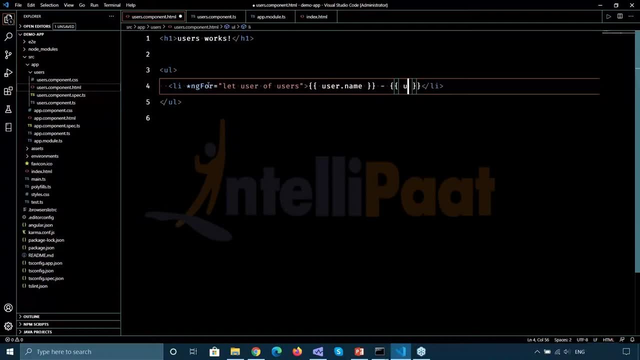 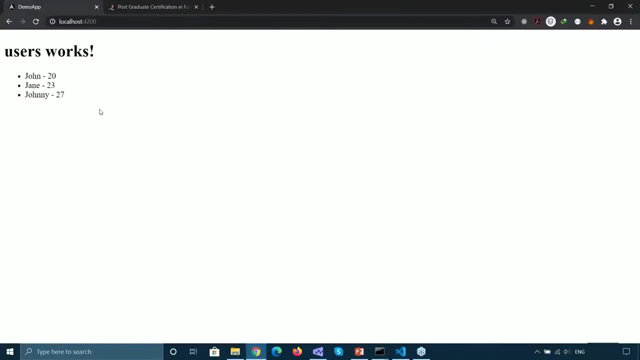 are going to tell the angular compiler. replace this with the dynamic value that I'm asking you to do. So each I save this now and I go back. as you can see, It's showing me. It's showing me the name of the user as well as the age of the user here. 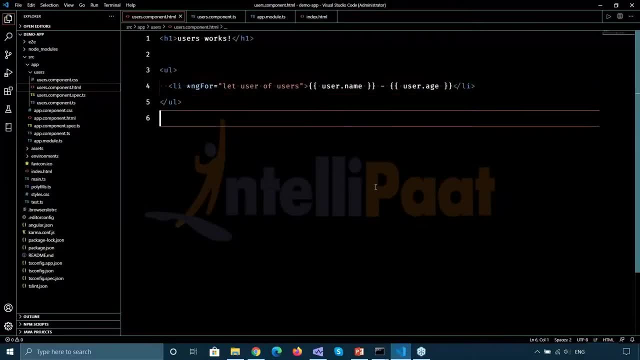 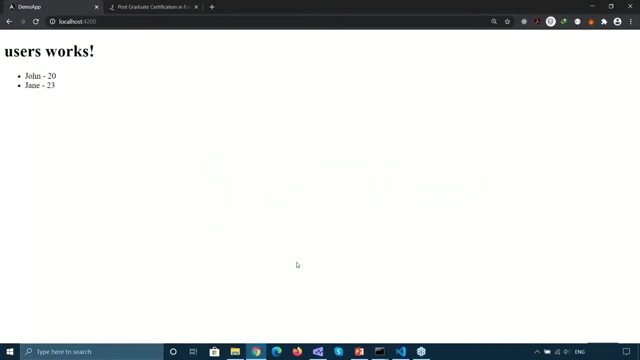 Of course I can change the structure in any other way I want to, but that's the first way I can do it. If I add a new user, remove a new user- Let's say I remove this- I don't have to make any changes to my code. 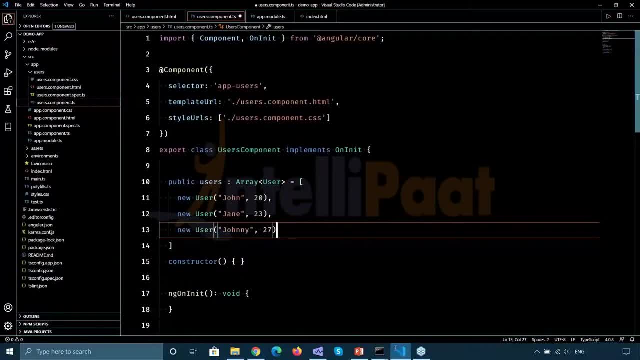 It is will be done by the angular compiler automatically. So, as you can see, it's quite dynamic. So that's one of the ways that angular directives help us. So with that, let's take a look at the third kind of directive that we want to take a look at, which is the attribute direct. 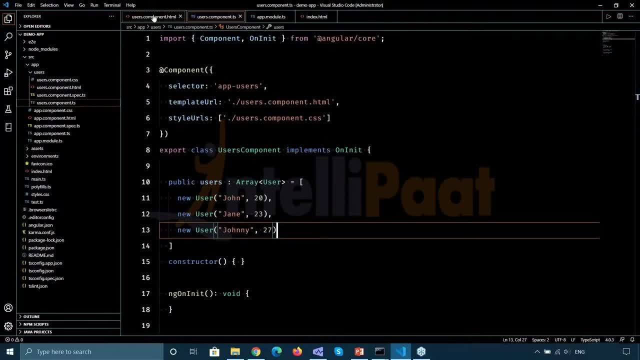 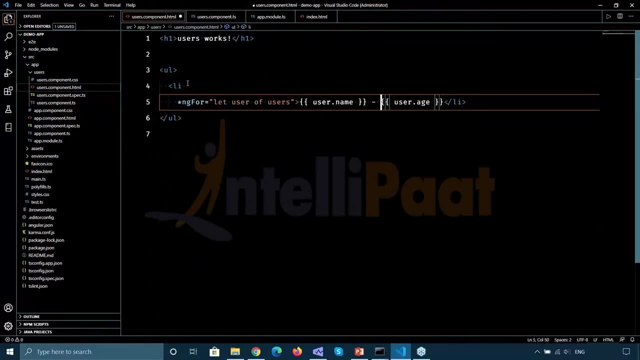 So now that that is done, I want to go back to my users component. I will drop this on a new line so that you can see it clearly what it's doing. This is to be dropped on new line as well. And again, angular compiler is quite sophisticated. 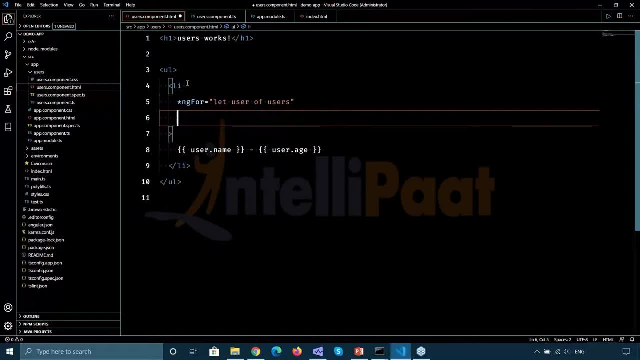 It can take a look at this and understand all of this. and now I want to add another attribute. This is going to be an attribute directive, So I want to apply some style conditionally. So this is going to be ng style. And here I can type in some JavaScript code inside a object syntax. 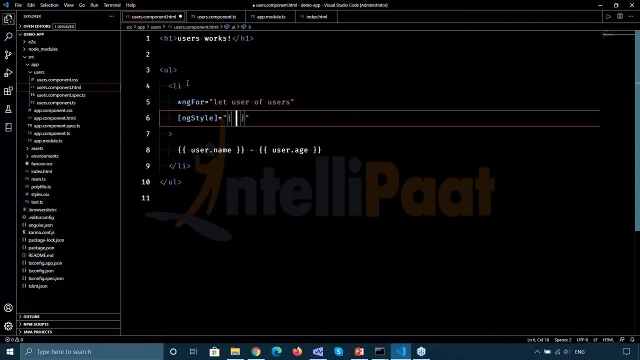 The key of the object is going to be the style I want to apply, and the value is going to be generated dynamically, So I want font weight to be applied. The key is already given, which is font weight, and the value is going to come as such. 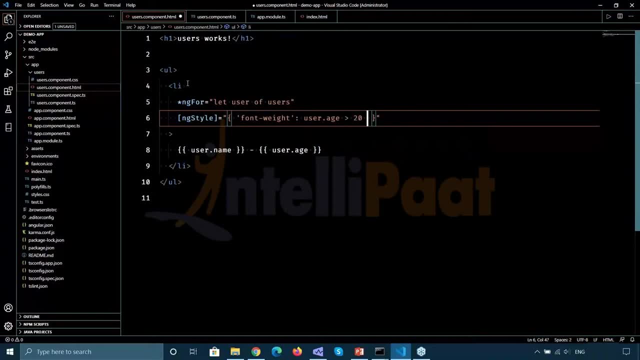 So if the user's age is greater than or equal to 20, then it's supposed to be bold question mark, and for bold I have to type in the correct words and otherwise nothing. Now, if I save this, I'm going to run into an error. 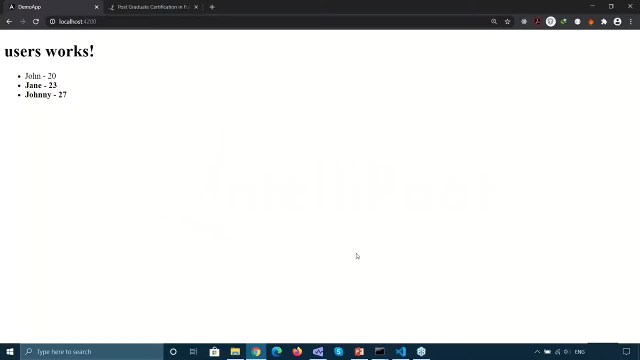 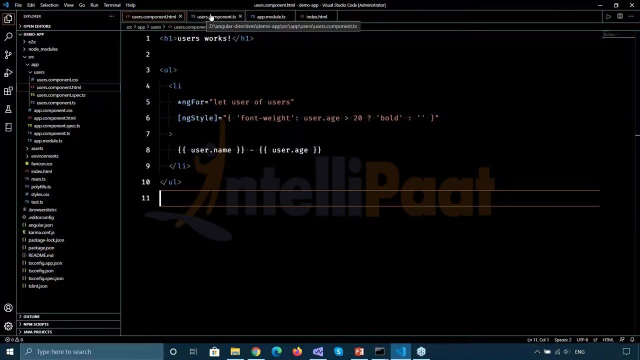 and you'll see that in a moment. So it works right now and if I go back to my code, this is applied correctly as well. So thankfully we didn't run into any errors. I go back to my code here. Sometimes what happens is you would have to. 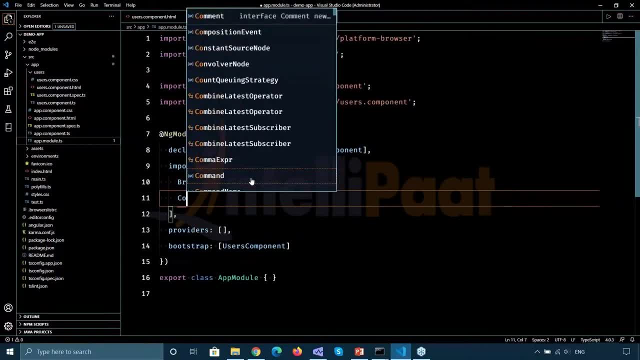 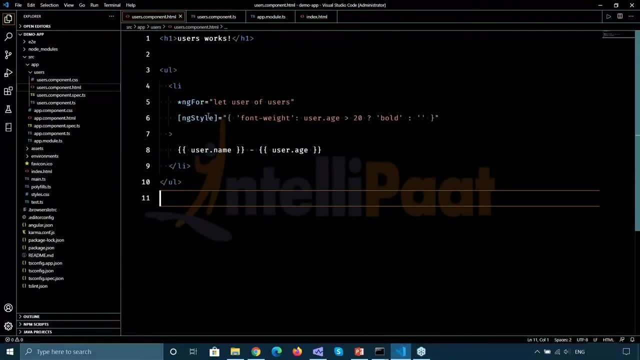 import something called a common module. I'll just import it here, common module, and save it, and this works as well, If I were to go back to my code. so this is working and you can see that the data that we had provided to our users, component John, is the only one whose age. 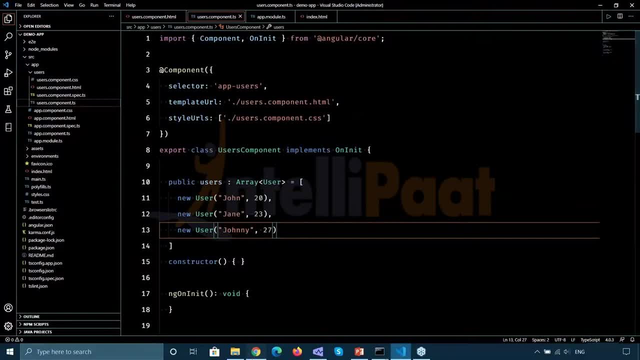 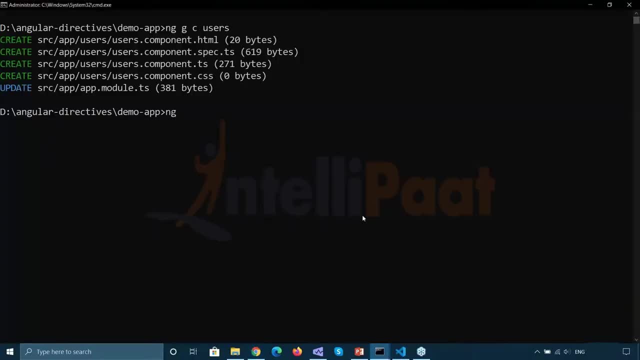 is equal to 20 and not greater than 20.. So John does not have a bold typeface. So with that now we've come to the final one, which is our generation of directive. So I will generate a directive. call it highlight. I will press enter again. 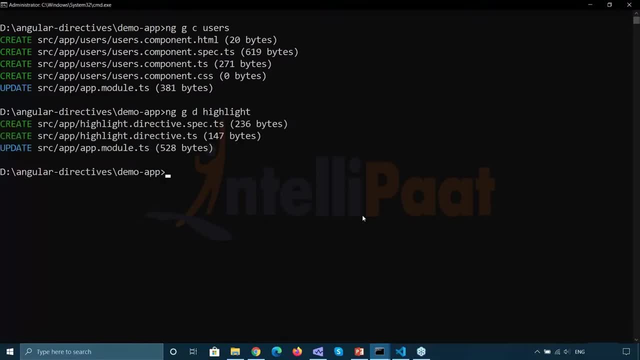 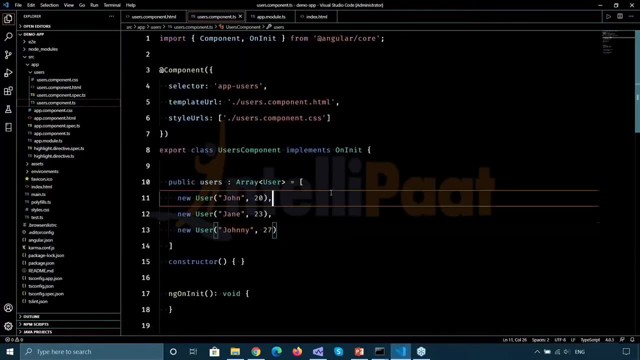 This will take a little bit of time and it will generate three files. So it has already done that. So it generates two files and it adds a new directive to our app dot module. So if I were to close all of this, look at the modules. 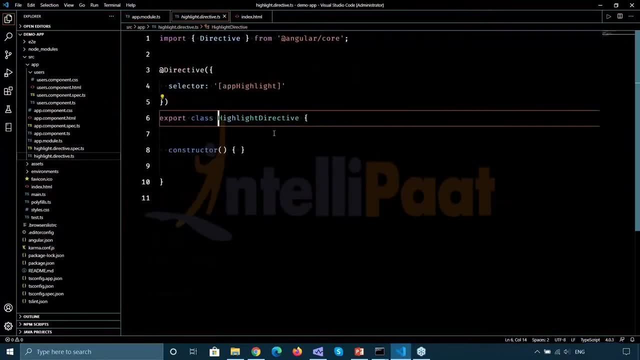 I have, and it has already imported the highlight directive. Now here's when I want to make the changes. So in the directive, what I want to do is I want to add an element reference. So this is going to be imported from angular code and, as you can see, 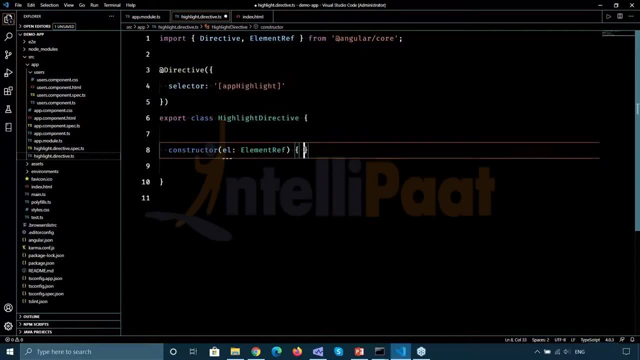 the selector name is app highlight. So this is what the directives supposed to look like. Now, when the directive is applied, I want to get the native element in the style tag in the style of the native directory. I want to change the background. make sure that you're typing it correctly. 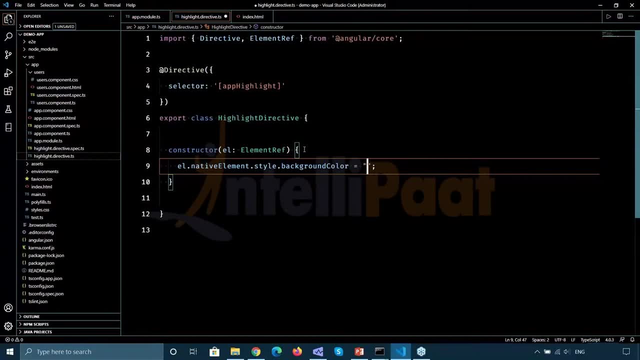 The name is really important here and I want to change the background color to, let's say, yellow. save this, So let's hope no compilation errors have been given to us so far and we have none. That's good. I have to go back to my template here. 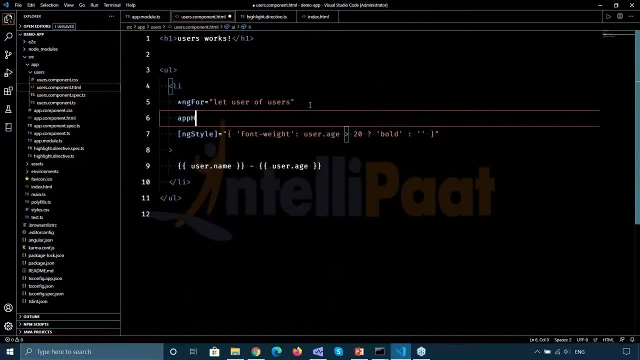 If I were to type in app h-i-g-h-l-i-g-h-t. If you take a look at the code right now it's showing it like this: save this, go back. and now it's showing the app highlight again. This could be applied with a particular course. 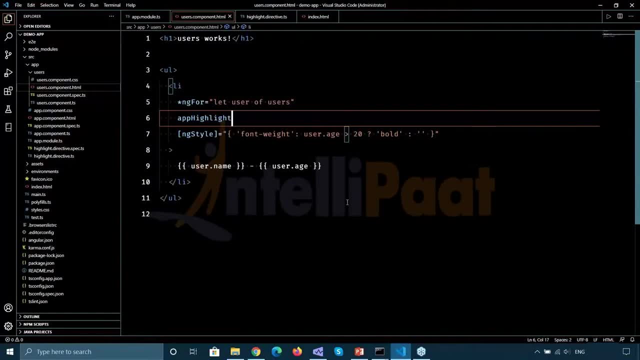 of conditional statements, but we can take a look at that later on. So we have discussed all four kinds of directives. Just to recap, we have taken a look at a component. We generated a new component named user component and we added that component into our browser. 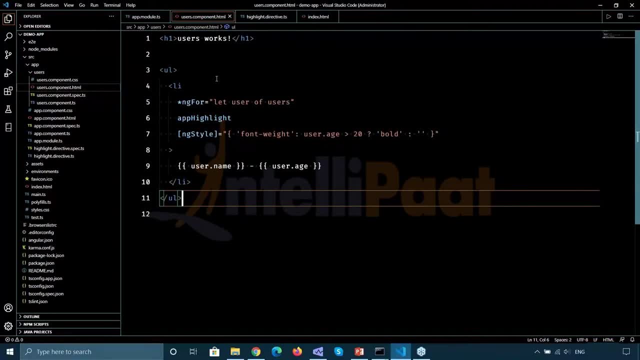 Then we have created another component named after creating the component. We have taken a look at the structural directive using ng4.. We have taken a look at attribute directive, such as ng style, and we have taken a look at custom directives, which is app highlight. 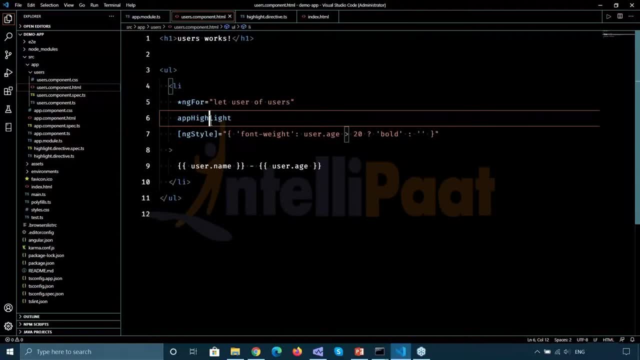 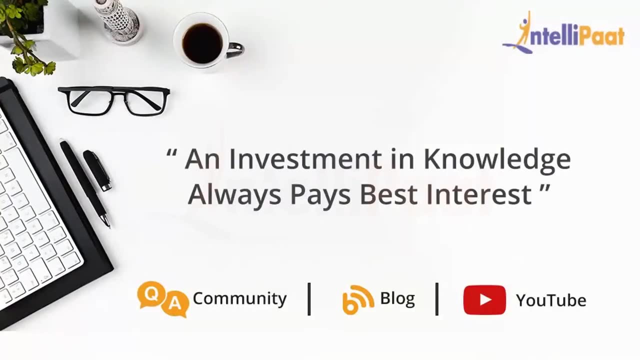 We can do a lot more with directives- too much that we can't cover here- but that's how this works. So with that, let's take a look at what else we have. So an investment in knowledge always face The best interest is a quote that always helps me. 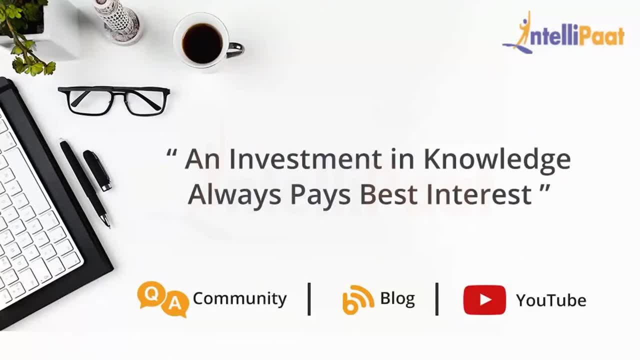 when I'm learning something new. keeping that in mind, If you want to learn something, if you run into some errors. you are learning something new, new technologies- and you run into some error, some exception, some code issue. You can take a look at our community site. 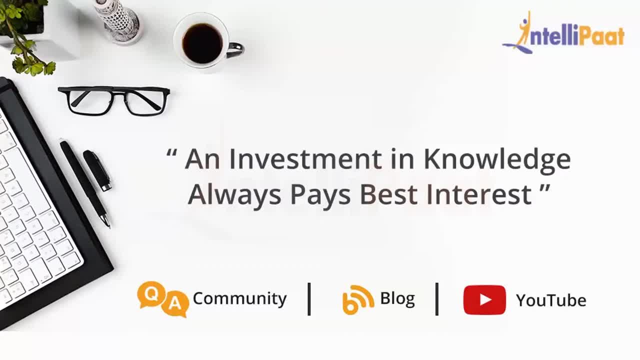 intellipaatcom slash community, where we have a group of people who are, such as you, like-minded individuals Who can help each other out and, in particular, technologies that they have an interest in, and you can help them out if you wish to. We also have a blog. 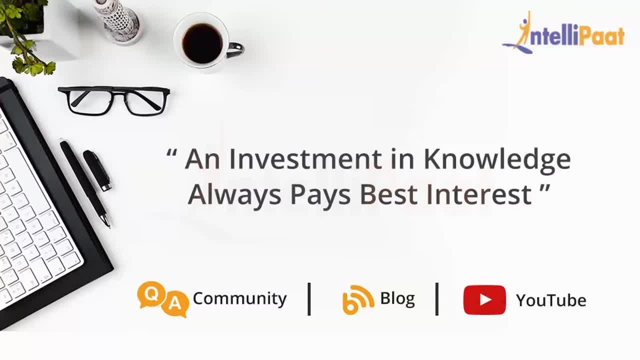 intellipaatcom slash blog where we publish new content regularly. The content ranges from technologies about about a web development, cloud computing, data science, machine learning, computer vision and all the new technologies. You can take a look at that as well. You're more of a visual person. 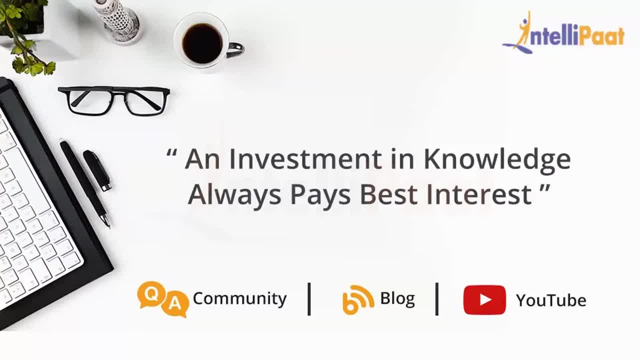 You can take a look at the YouTube channel that we have. We have a lot of free content there as well. You can take a look at those Free videos and upskill yourself, in case you don't want to take a look at a course. 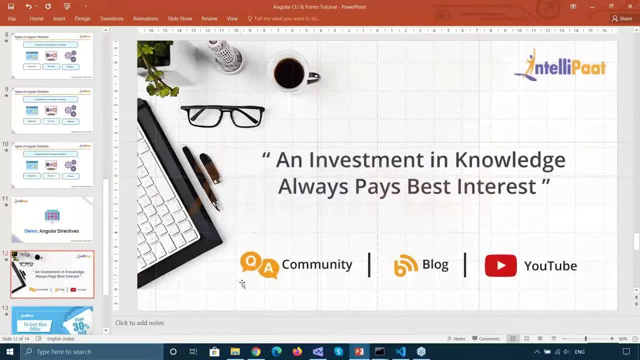 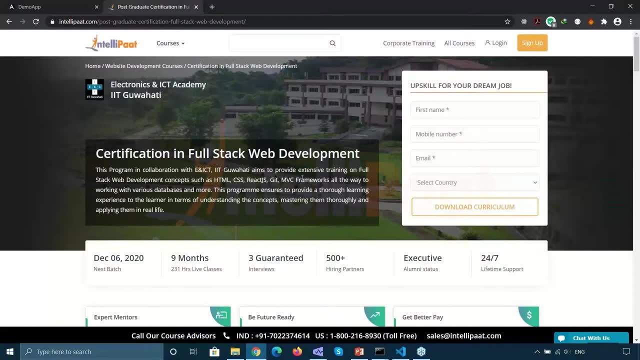 but you want to upskill yourself and get certified in order to get a job. We recommend that you take a look at the web development post-graduation course at our website. This is accredited by the electronics and ICT Academy in IIT Guwahati. 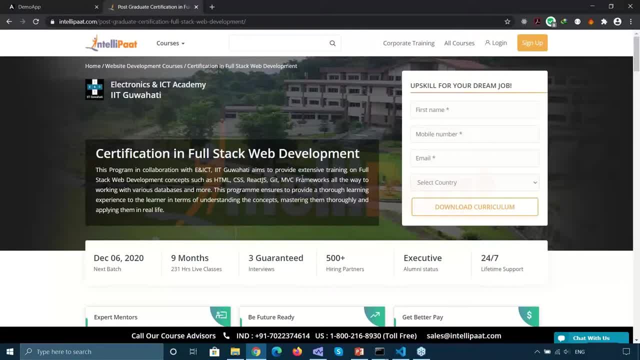 It's a nine-month course. The next batch is starting on 6th of December. You can take a look at all the features that we provide, ranging from 24-7 lifetime support, three guaranteed interviews and so on. You can take a look at the details on the page. 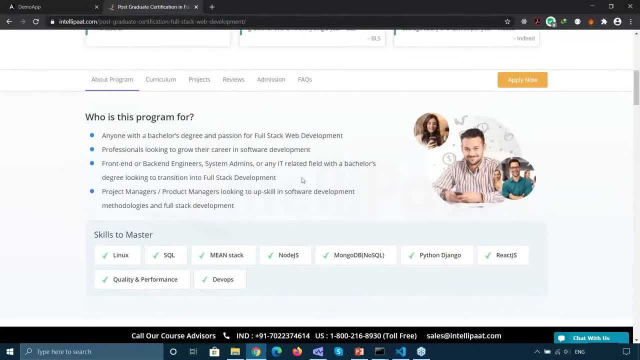 You can take a look at. who is this program for? What are the skills that you will learn, ranging from Linux, SQL, Mean Stack, Nodejs, MongoDB, Python, Django, React. So you learn a lot of technologies and we teach everything from completely grounds up. 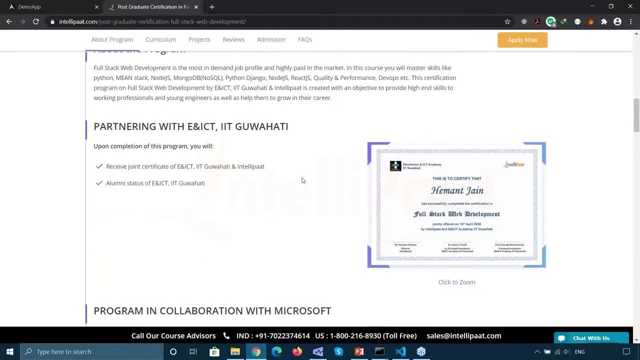 You can take a look at the course certificate. You can receive joint certificates from both IIT Guwahati's ICT Academy and Intellipaat, and you receive an alumni status of electronics and IIT Guwahati's, So you can take a look at these two certificates. 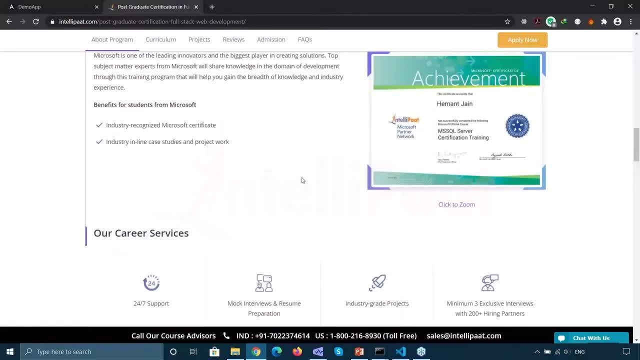 that you'll get. and you get 24-7 lifetime support. You get mock interviews and resume preparation, industry-grade projects and minimum three exclusive interviews. Now, industry-grade projects are really important here because you get to learn new things and apply it to real-world problems. 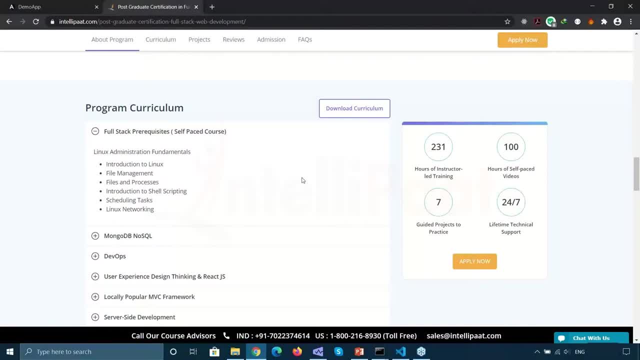 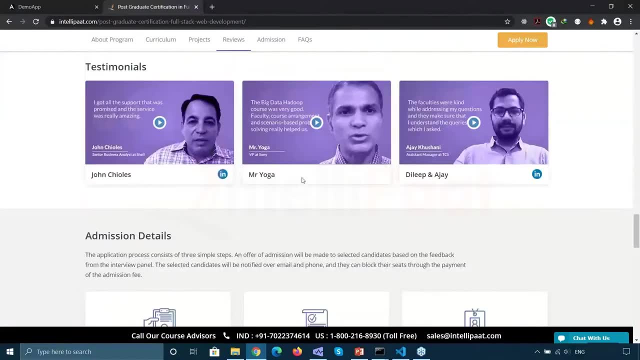 You can take a look at the program curriculum. We teach everything from complete scratch, So if you don't know anything, you can still join. You can take a look at the projects that we cover: testimonials. this is one of our highest rated courses. 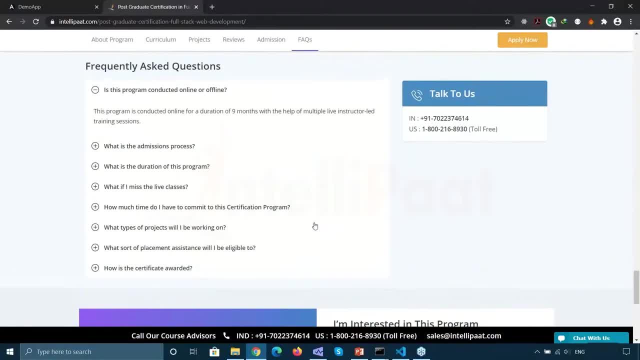 Take a look at the admission details. If you have any questions, you can take a look at the FAQs. In case your questions are not answered in the FAQ section, we recommend that you can take a look at another resource, which we'll show you in a moment. 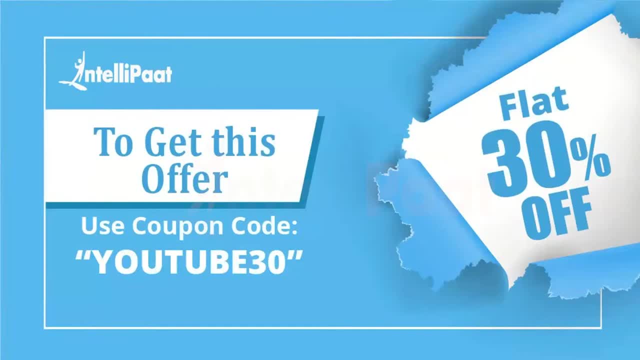 But before that, thank you so much for joining us. Here's a coupon code for you: YouTube 30.. You can take a look at it and get 30% off on any course that you want to buy off our site. This code is valid for a limited amount of time. 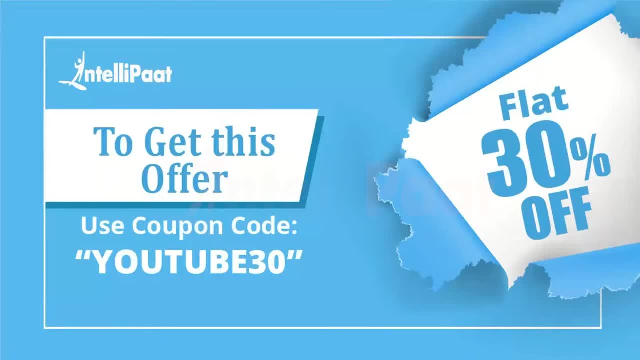 So we hope you make use of it as much as you can. We hope you make use of it as quickly as possible. With that, we've come to the end of the presentation and we have a few numbers that you can call in order to get more information. 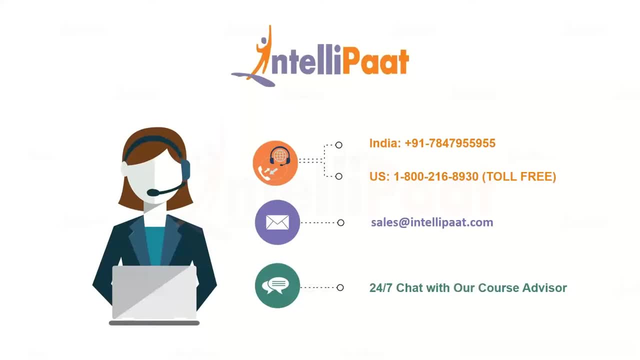 in case your questions were not answered in the FAQ section, or if you just want to discuss something about your career trajectory, Our course advisors are there to help you out 24-7.. If you're more of an email person, you can contact us on the emails listed on the screen.